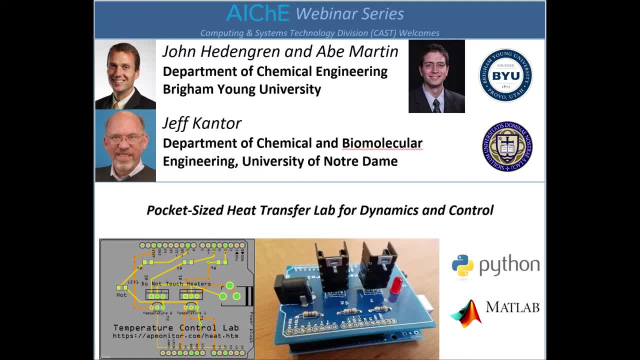 And I'm an associate professor here at Brigham Young University and I do work in fiber optic monitoring, unmanned aerial systems, automation of drilling and other upstream infrastructure. And then we have on the line as well Abe Martin. He's a PhD candidate here at Brigham Young University in my group. 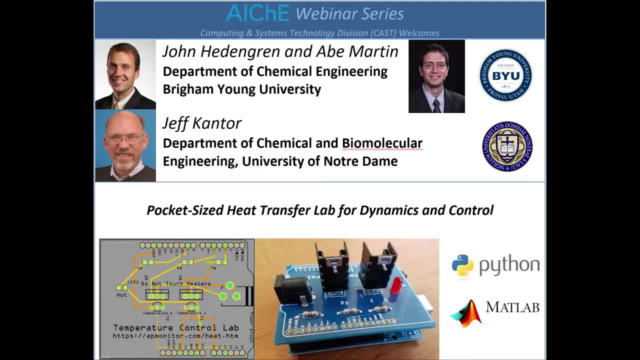 He focuses on aerospace design and control, particularly with aerospace High altitude long endurance aircraft, And he recently completed an internship at Air Force Research Labs with a focus on computer vision aerial vehicles, And he has prior work experience at Idaho National Labs, And he's going to be graduating in 2018, so if anybody knows of good positions that are available, he is currently searching. 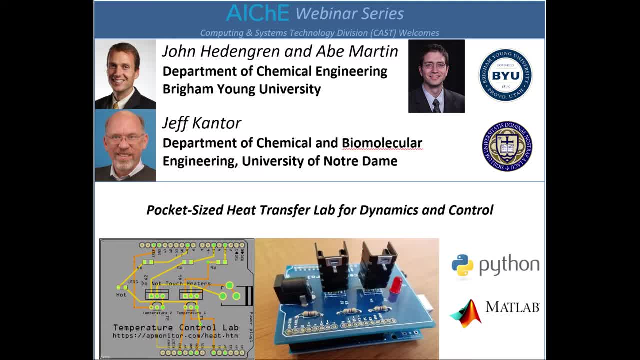 Then we have Jeff Cantor. He got his bachelor's from the University of Minnesota. He has an MA and PhD from Princeton University. He joined Notre Dame in 1981, and he was the vice president and associate provost and then became vice president for graduate studies and research at Notre Dame. 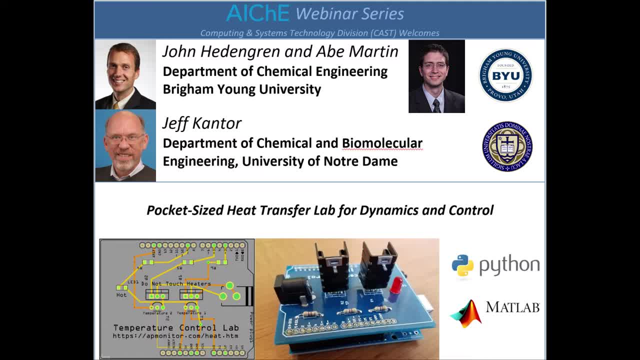 He's currently a professor in the Department of Chemical and Biomolecular Engineering, And Dr Cantor is interested in analysis and optimization of integrated financial and process operations using methods of stochastic control, convex optimization and quantitative finance. And so with that we'll go ahead and get started on the presentation. 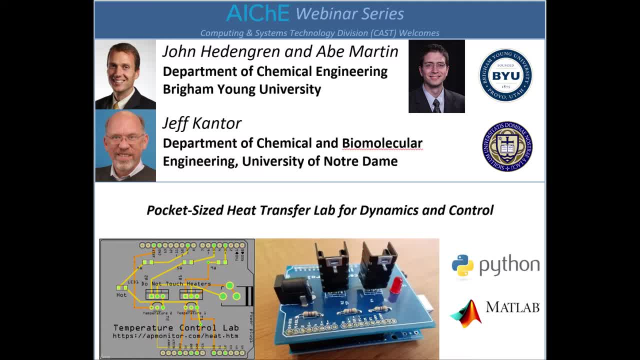 And I'll go ahead and we're just going to be doing a brief overview of the lab today, And then what we'll do is give a brief demo. Let's see, I've got to figure out how to swap presenter. Okay, Okay. 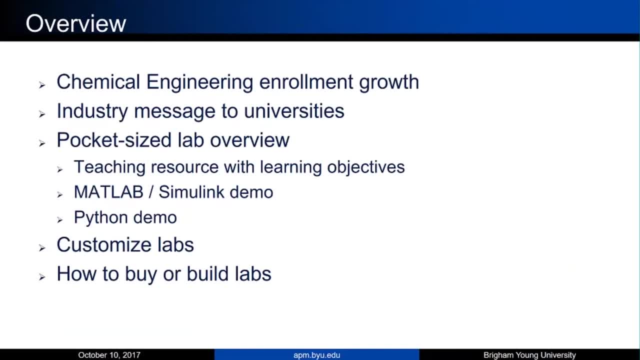 So we have introduced us. Here's the overview. We're going to talk a little bit about chemical engineering enrollment growth. A lot of us are interested in this topic, of these small modular labs, just because of the enrollment growth and the way we teach, process dynamics and control. 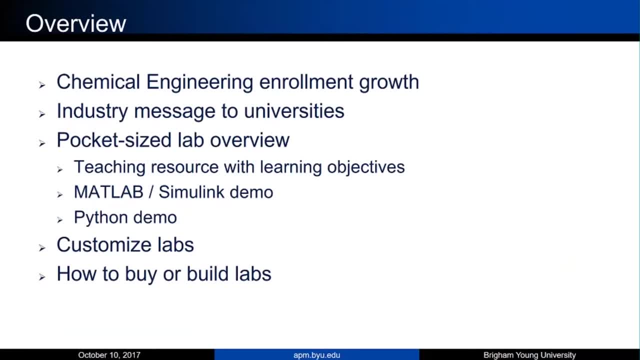 Then a little bit about a recent industry message to universities, a survey from an industry and academic alignment, And then we'll give the pocket-sized lab overview and talk about some of the teaching resources that it provides, with a link or some demo with MATLAB, Simulink and a Python demo. 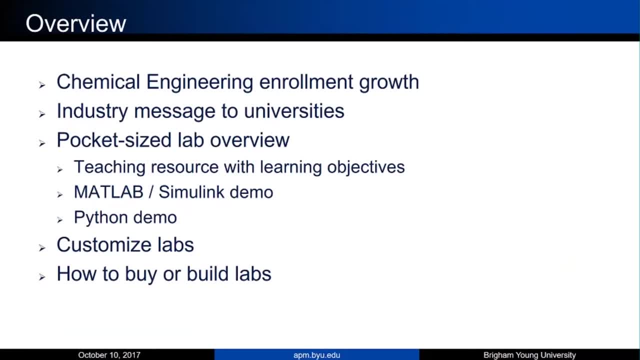 And then Jeff is going to talk about how to customize the lab. He's at Notre Dame and he's taken this lab and has some plans that he'll share. And then the final thing is how to get in on the bulk order that we're submitting. 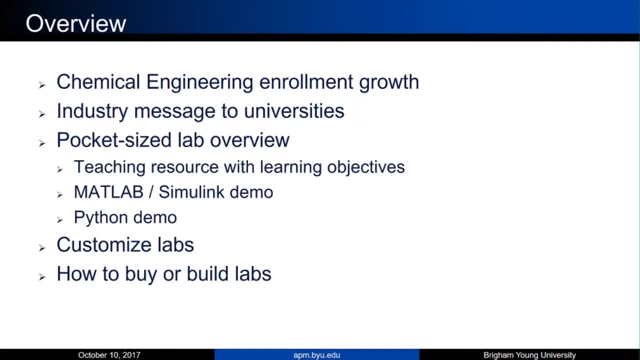 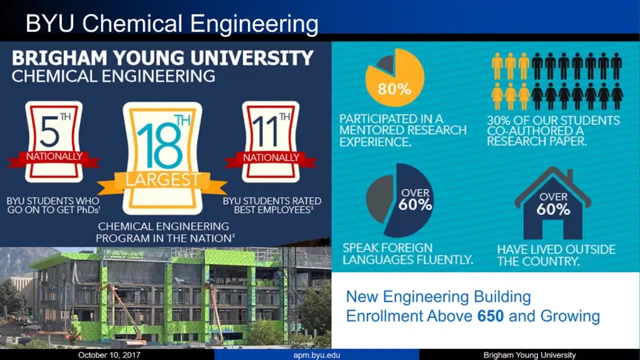 And we've already had a number of universities that have expressed interest in that. Okay, So a little bit about Brigham Young University, 18th largest chemical engineering program in the nation. We have an enrollment above 650, and it's growing. 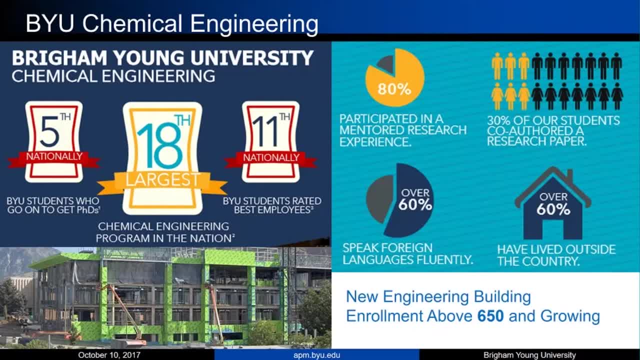 And, frankly, we're struggling a little bit with how to give the same type of classroom experience with classes of 120 students, versus what we had just 15 years ago with 4,000 students, And so it's causing us to innovate and change what we do. 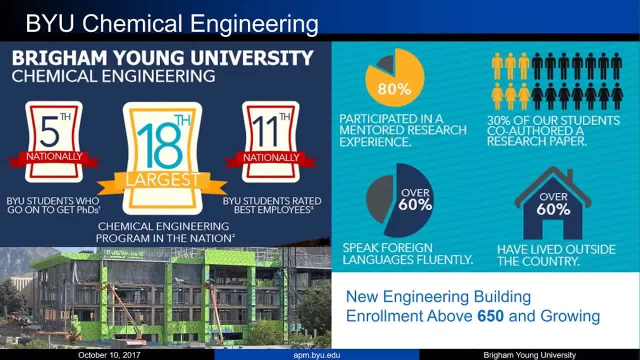 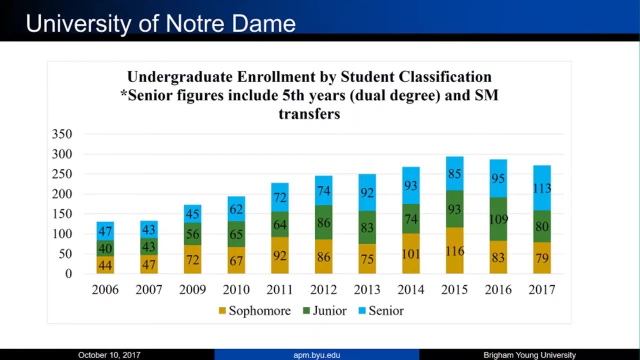 On the bottom left is our new engineering building, So if you hear any construction noise in the background, it's because that's being built right now. So that's part of the expansion that we're currently dealing with. Jeff, do you want to say a little bit about Notre Dame as well? 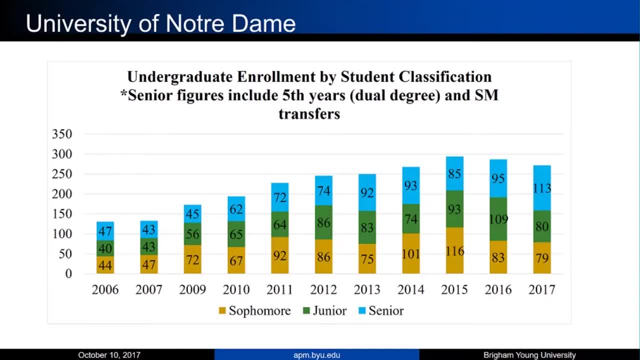 Sure, I think we're seeing the same phenomenon that you have and others have at their schools. We've seen growth. This slide just shows our growth since 2006.. We've over doubled and then, I guess, like you, we're struggling with larger class sizes. 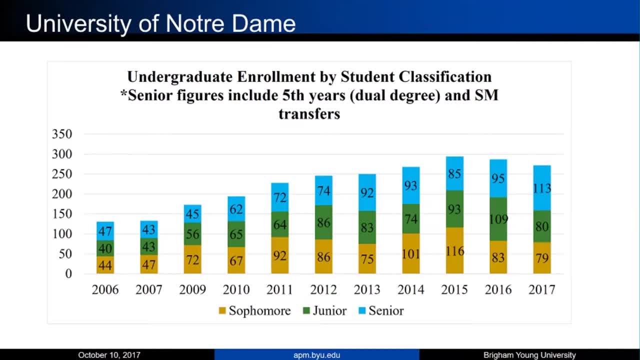 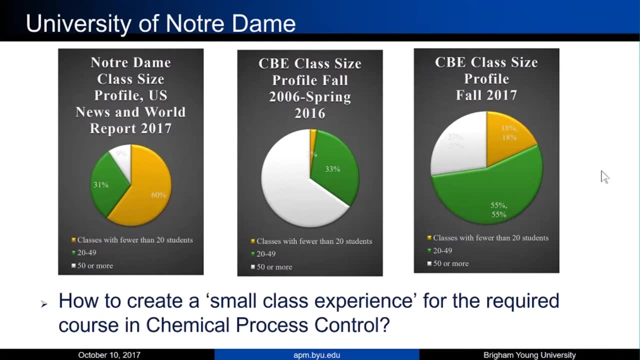 And how do we offer a lot of experience for students when they come in such large groups? Okay, great, If you just go ahead. one slide, Yes, this kind of- shows a picture of what's happened to our class sizes. On the left is a picture of class sizes. 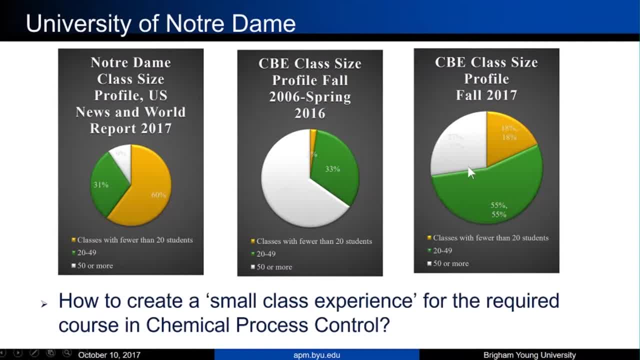 The class size profile at Notre Dame as a whole. the large gold is our classes of fewer than 20 students. The predominant number of classes on our campus are taught in very small sections. We're very fortunate that way. The middle slide, though, shows what our chemical engineering program was like just a few years ago. 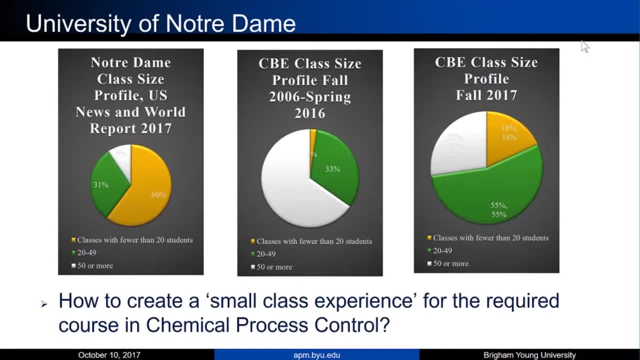 the white being class sizes of 50 or more. On the right, it's the result of breaking up some of our larger classes into smaller sections. So we've been able to address the issue, but we have a mandate. Our department has a mandate from the university as a whole to try to find better ways to personalize the experience. 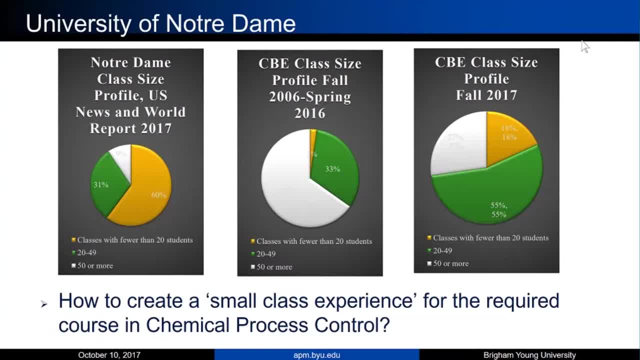 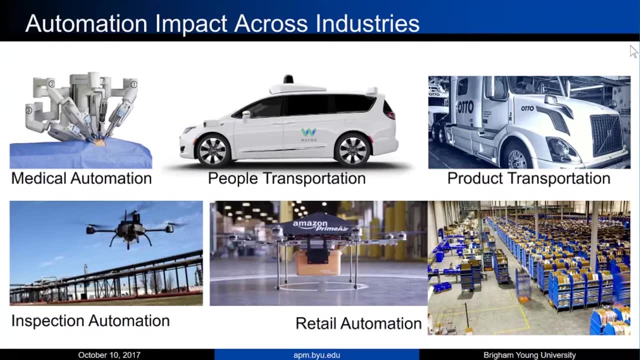 for our students and to provide them more of a small class environment, to the extent that we can. So the pocket-sized lab is my contribution to that effort. Great, Okay, and then a little bit about industry. You know automation. we all see automation as really affecting a number of industries right now. 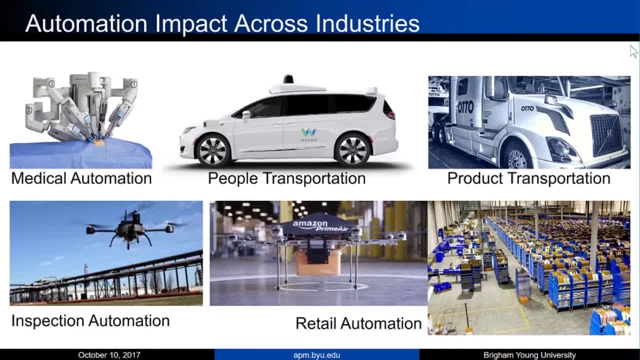 and there seems to be an increase in interest from industry on automation process control. those who understand dynamics You know we think about medical automation, people transportation, product transportation, inspection and then retail, One of the key studies in this area about transportation. 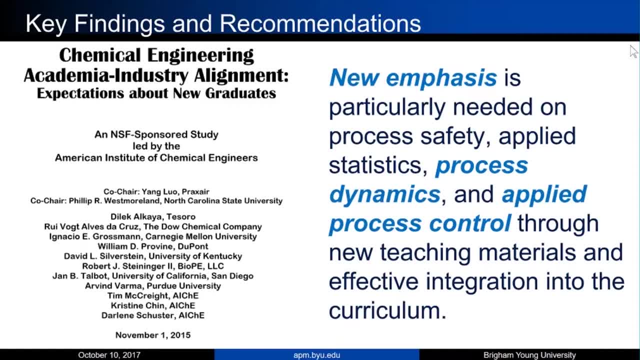 chemical engineering, how we teach, and also some feedback from industry was given by this NSF-sponsored study listed there on the left, And one of the key outcomes of that study was that they recommended new emphasis is particularly needed on process safety, applied statistics, and then I've highlighted there process dynamics and applied process control. 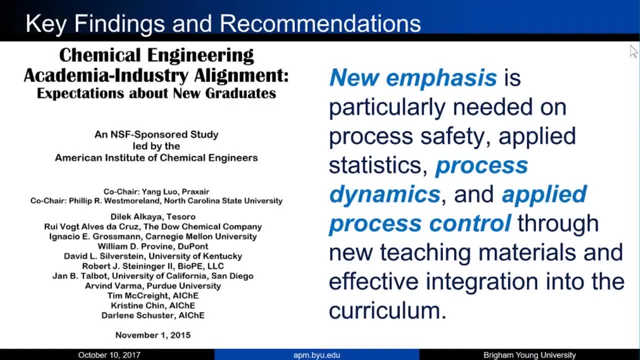 Through new teaching materials and effective integration into the curriculum, And so we've been given a mandate from industry. As Jeff mentioned, they're trying to personalize and make these class sizes, give each student an individual experience, But sometimes we struggle with only having one or two larger labs that students have to go in and schedule and find time to use. 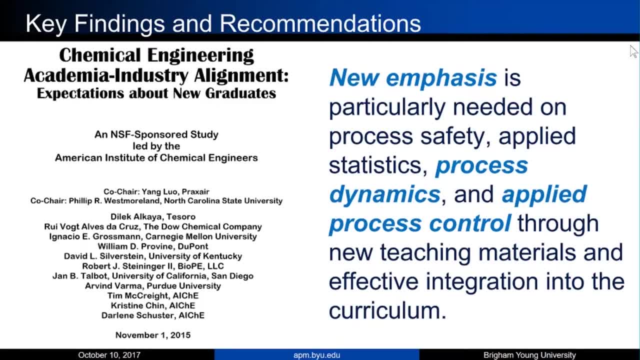 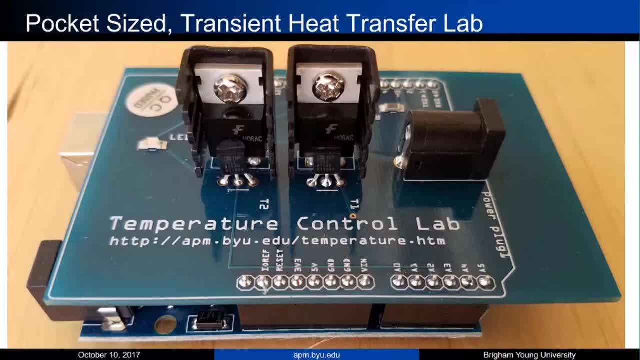 So we're trying to develop this lab To meet this need that's currently there with increased enrollment. So I'll turn it over to Abe now- Or Abe really is to blame for a lot of this, Because he helped to develop this lab originally. 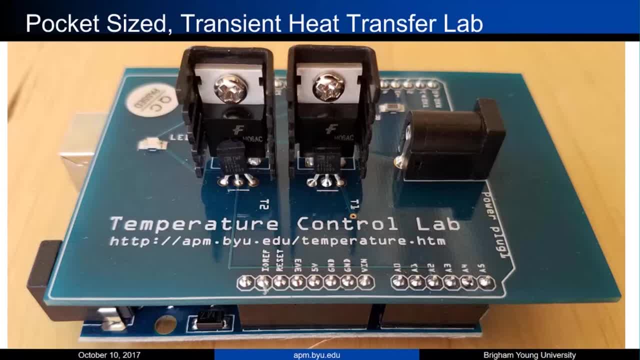 So I'll let Abe talk a little bit about what he's done with this. Yeah, so I'll just give a brief overview of this lab, Kind of some of the things we've put together and some of the history of what we've done here at BYU. 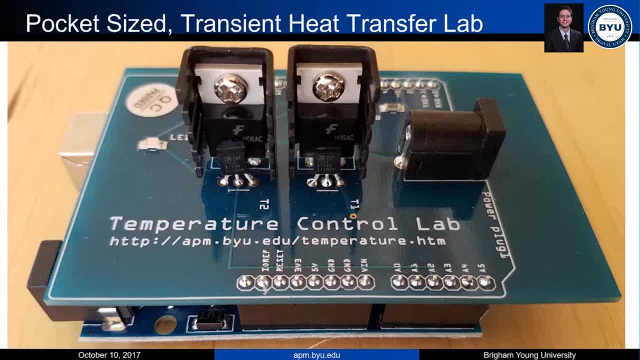 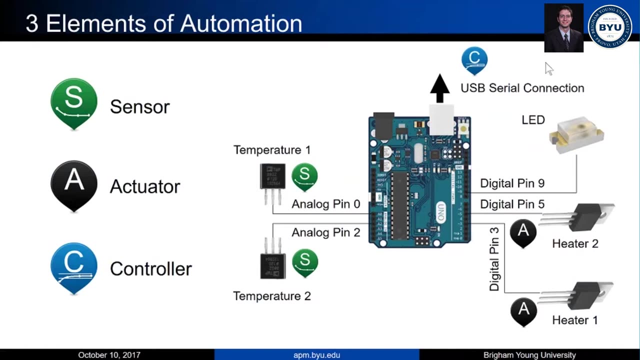 With this small modular process control lab. So there's an image of the lab we have right now. So in any automation control lab you need three things. You need at least a sensor, an actuator and a controller- A sensor to sense the environment. 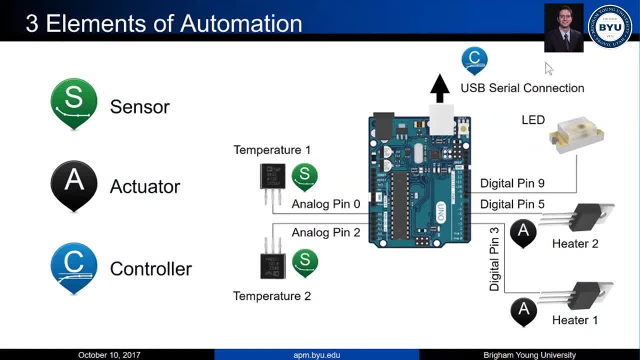 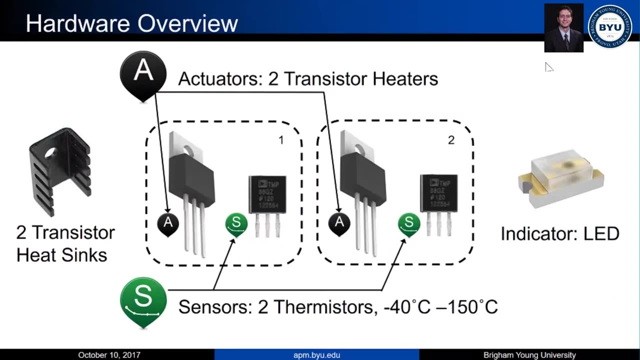 The actuator to affect the environment And the controller to go between those Sensor input and control, Controlling the actuator to affect the environment in the way you want it to be. So in the case of this modular process control lab, we put together 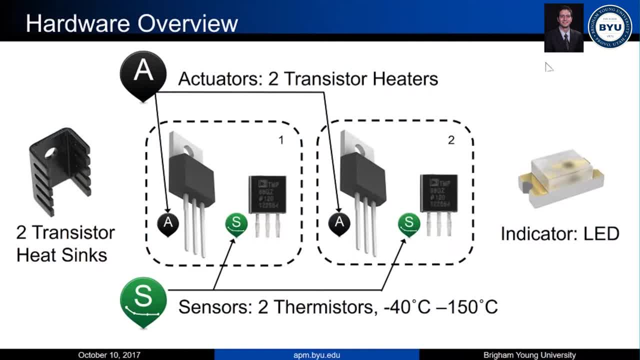 The actuators are two transistor heaters. Sensors are two thermistors or temperature sensors that sense the temperature of the transistors, So we're able to control the voltage going through these transistors, Which in turn affect the temperature of the transistors. 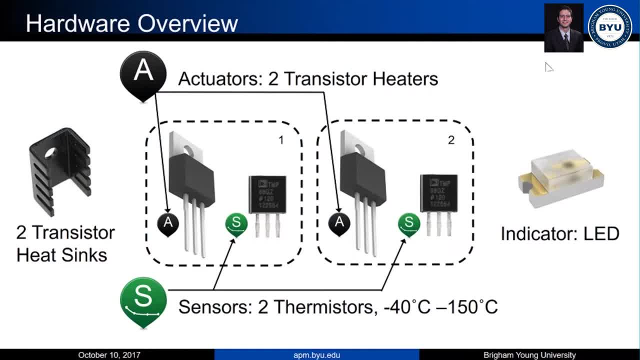 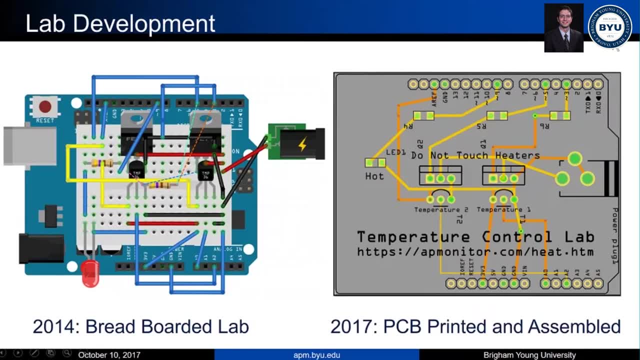 And measure that, Set up a control loop Just on a small board there. So if you look on the left there, You can see the diagram for our original breadboarded lab. Started out with the sardino boards, Put a small breadboard on top. 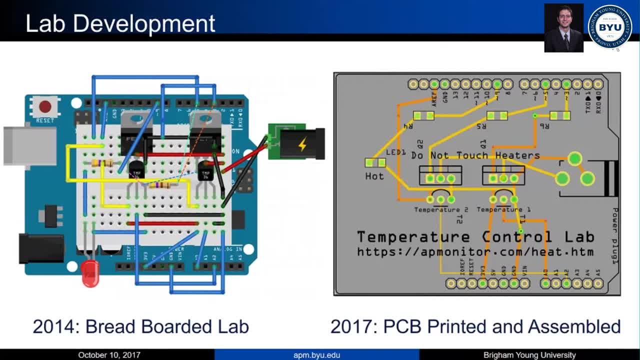 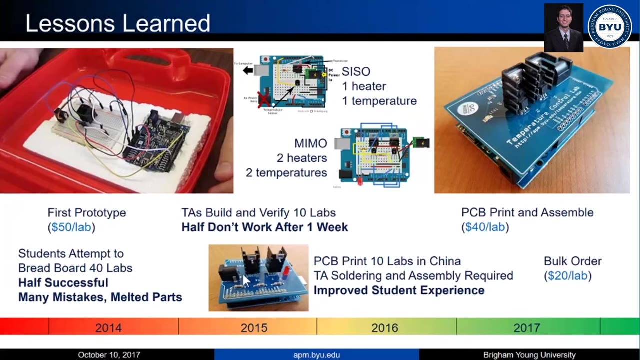 And wired together. the process control lab Progressed since then. We've come along to We're using a printed and assembled PCB board, Which is much better at this point. Go down to the next slide. See some of the lessons learned. 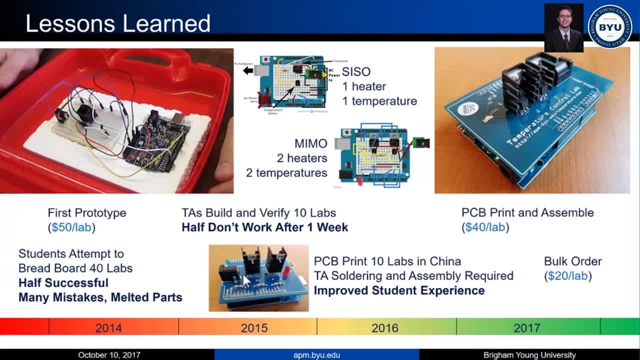 The left corner, there in the red box, See the original prototype I built of the lab. Took quite a while to put together, Designed the circuit. The first year we tried to deploy these We attempted to have the students put together the lab. 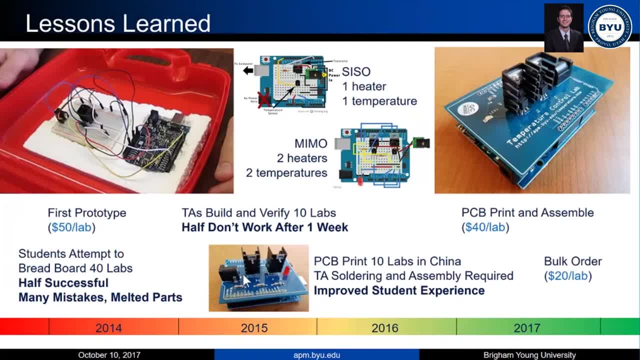 Breadboarded themselves. That didn't go over very well. Turned out that probably less than half of the students were successful in correctly putting together the lab. That led to a lot of problems later on when they were trying to go through the lab exercises. 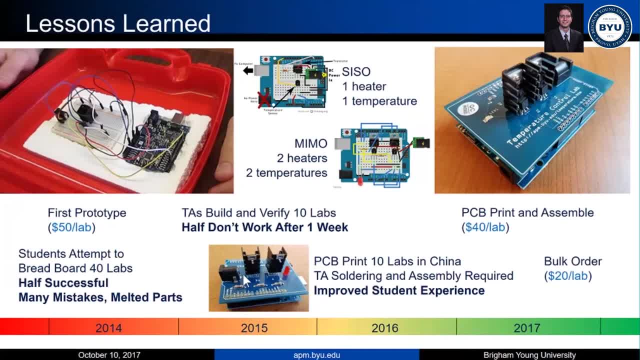 That being a safety concern as well. Some people short circuited their boards, Had some parts melted, Some fire hazards, Safety hazards. The next year we tried something different. We had the TAs put together the lab, Or put together just ten of the lab kits. 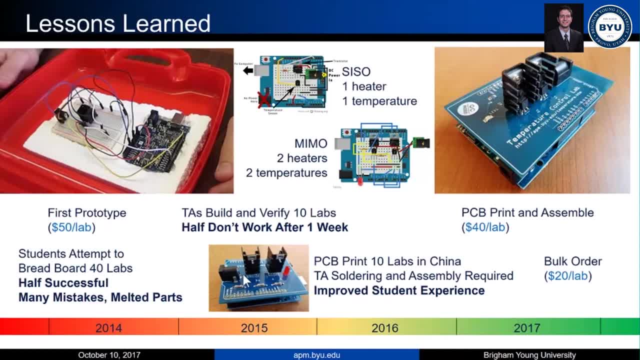 And left those in a controlled environment in the lab, Verified that each of the ten would work. That was a little bit better. We find, though, after a week or two, that many of them stopped working. People would move around And jostle wires. 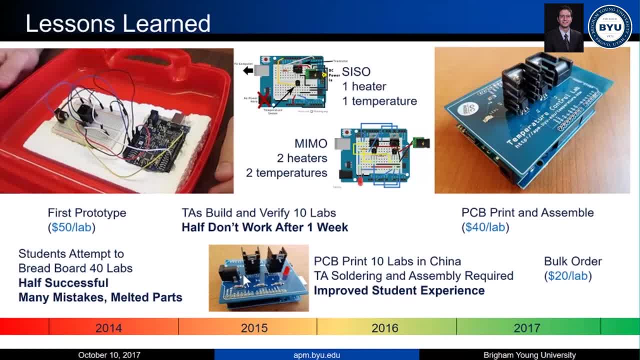 Wires would come loose, Parts would come loose, Things would get lost. That wasn't ideal either. From there we moved on to having the PCB boards printed To eliminate the problems that we had with wires. That was much more effective. First iteration with that we had TAs put together the lab. 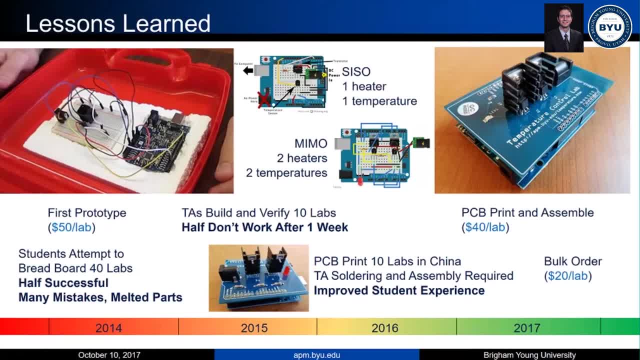 Soldered it together. That worked fairly well. It was pretty time consuming for TAs, though, To learn some new skills Soldering. In our most recent iteration we've been able to have the entire lab, The entire shield that goes on top of the Arduino. 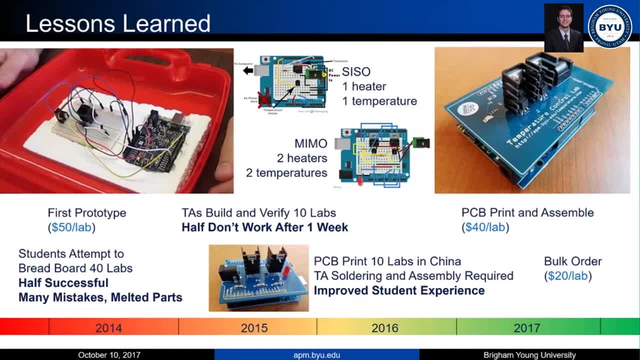 To be printed out and assembled in China. That's been working out very well for us. So we have the complete lab. We don't have to worry about any quality control issues And put that on top of an Arduino, Plug it in. 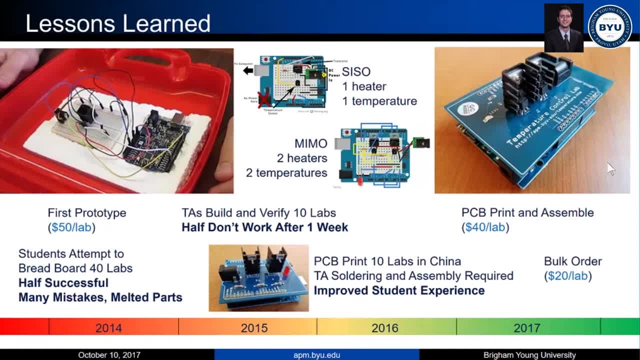 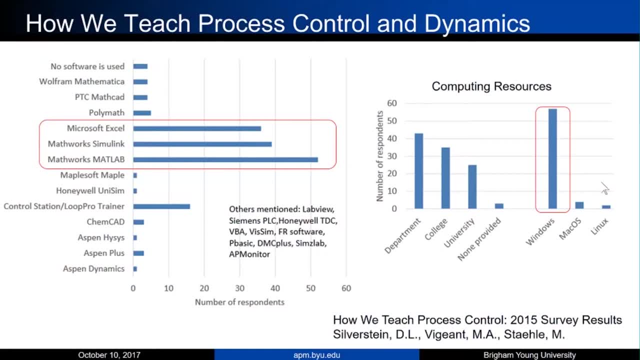 And they're good to go. So that's what we've been able to do. So that's what we've been able to do. So that's what we've been able to do. Okay, Thanks, Abe. So I'm going to talk just a little bit about how we teach process control in the US. 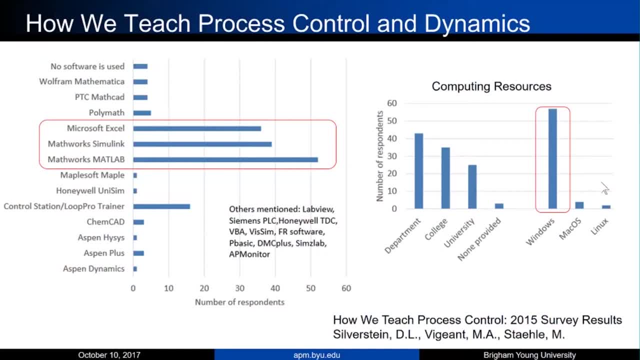 This was a survey that was done in 2015 by Silverstein and others. They surveyed process control and dynamics professors And found out that we largely use microcontroller, That we largely use Microsoft Excel, Simulink and MATLAB. At BYU, we've recently moved over to Python. 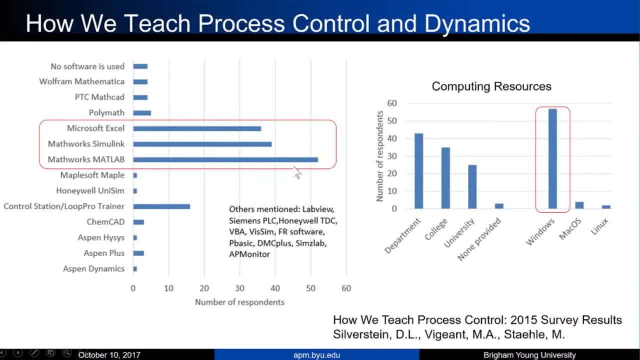 And a number of professors I've talked to have mentioned that there's interest in porting to Python as well. And then the other thing is computing resources. Most said that most of their computer labs are Windows based, Although many students their personal laptops are Mac OS. 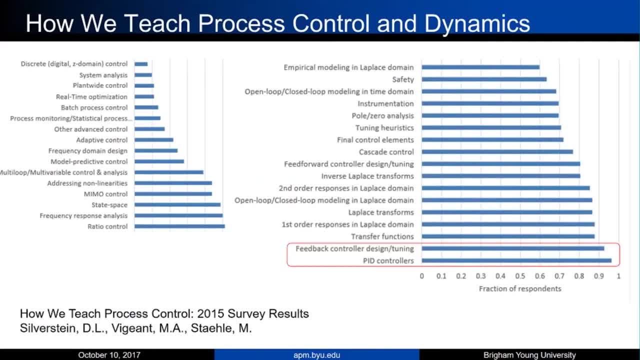 So they're using a lot of Linux as well. This is how we the subjects that we cover in process control. This was from the survey And this is the fraction of respondents that you can see there, So the length of the bar you know. for all that responded. 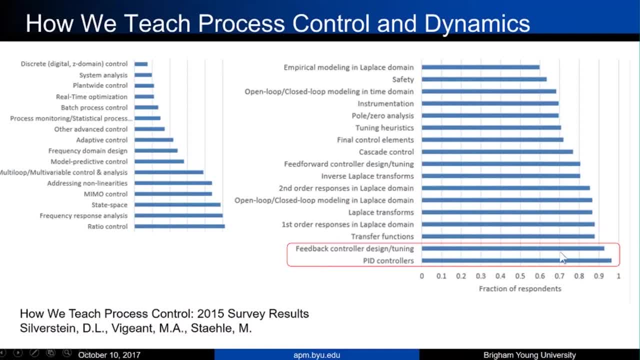 That's the fraction that covered that topic And this lab really addresses. you know, many of these topics. You can use these to develop modules That reinforce many of these topics, But the two primary ones are feedback controller design and tuning PID controllers. 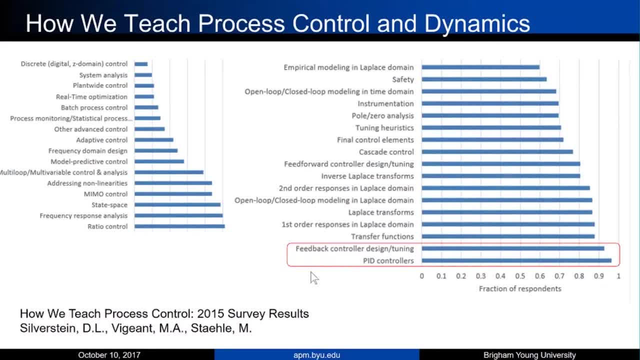 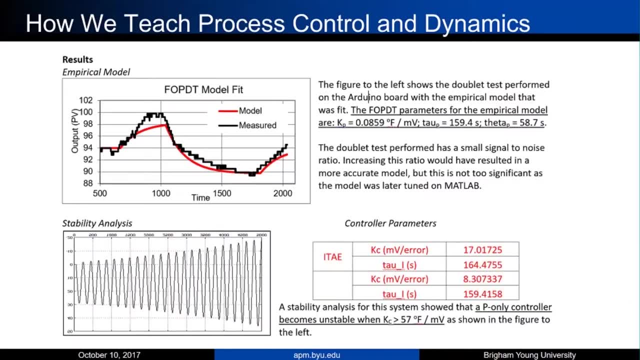 There's also parts of it that you can do with modeling dynamics, Which are things that industry said were very important for students to understand. This is a student report. I got permission to share some of this from the student And he you know, so this is an example of what a student might do with this lab. 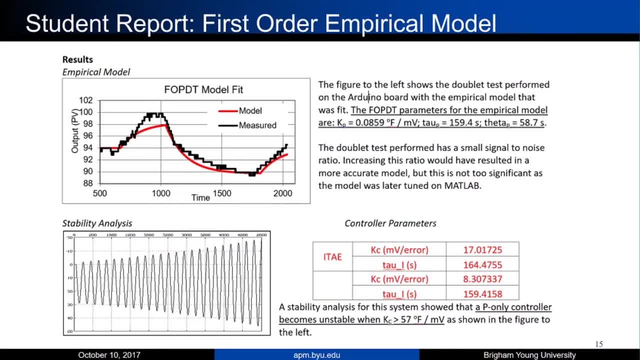 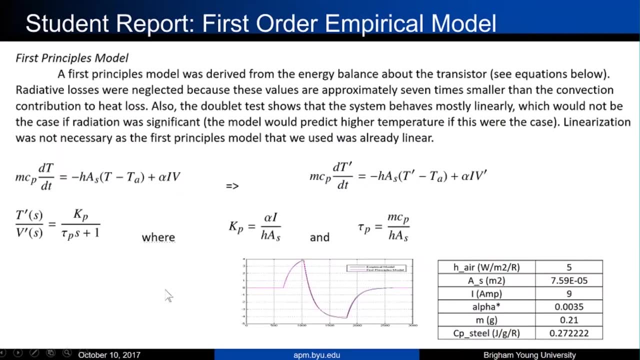 They would collect data, fit empirical or first principles models And then develop PID tuning parameters from that, Maybe do a stability analysis- As you can see here the stability analysis- they verified that- And then developing a first principles model. One thing that students are very familiar with is how to develop differential equations. 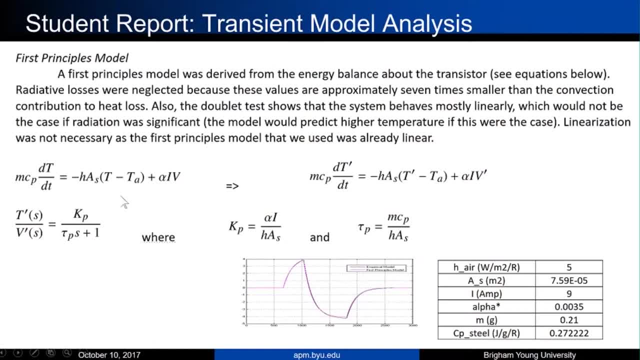 You know transient analysis And you know a lot of it up to this point has been very theoretical for them, Solving differential equations, And in this plot here you can see the empirical versus first principles models that align very well. 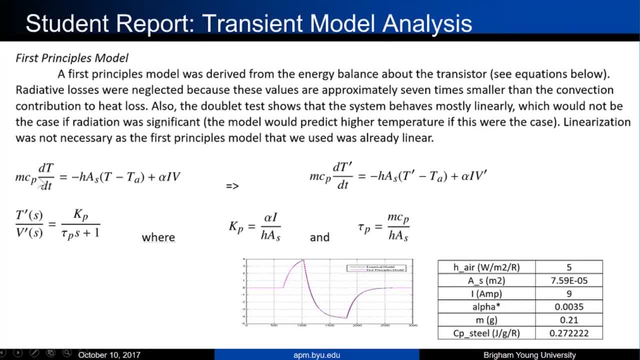 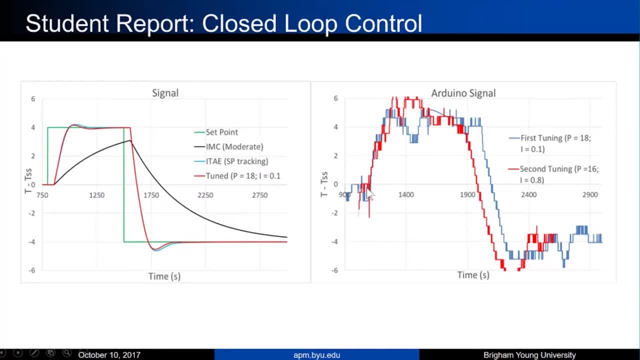 And the students are very excited about this. They can see that their theory is applying to practice. And then when they finally go to control the PID, they do it in simulation. So they try to get a certain amount of overshoot And they test some step changes in the set point. 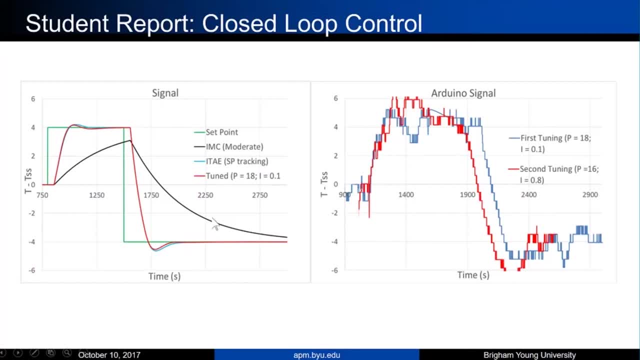 And they tune it. Maybe this is the initial tuning that was suggested, for example, by IMC, moderate tuning, And then they use ITAE And then they tune it further, And then they implement it in practice, And so this student probably didn't do big enough. step changes. 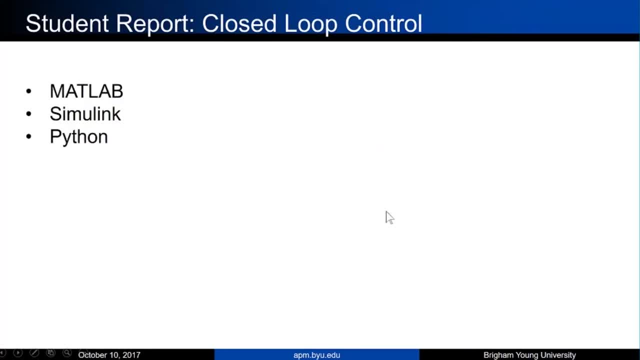 A lot of noise there in the signal But there's a. those are the you know the you know the you know the results of that student came up with. So I just wanted to first of all just give a brief demo on MATLAB and Simulink. 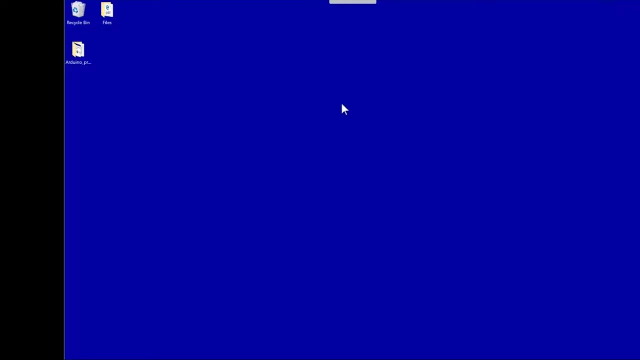 and just some of the things that are possible. with that, I just plugged in a new board, So this is like if the student were to get this, you know, out of the box, This is what the student would experience, And let me go ahead and just bring this over. 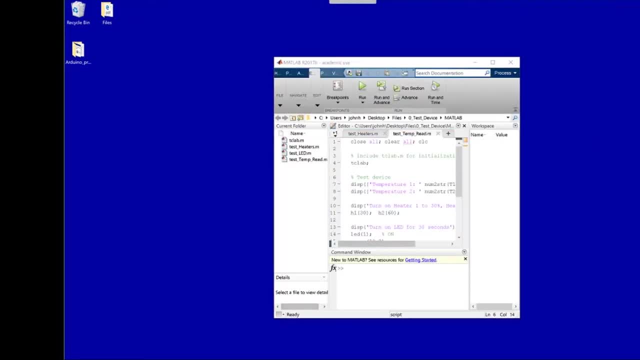 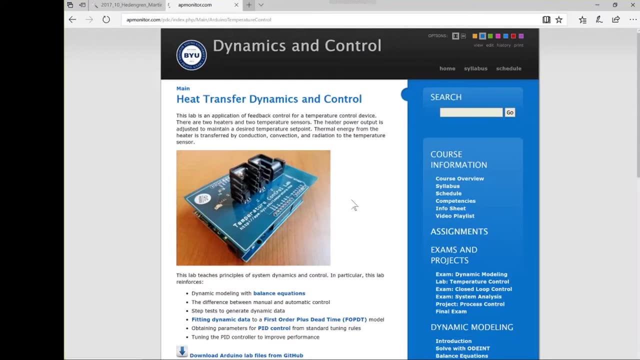 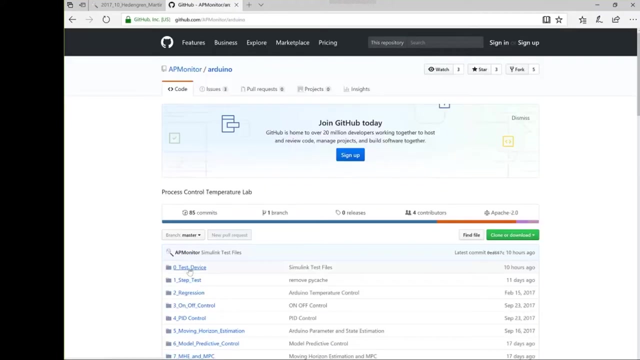 There's some example code that we have posted. So, for example, here is the lab website- A number of you have already seen that- And then there's a link here for download files from GitHub. And under the test device- under this folder zero test device- there's MATLAB. 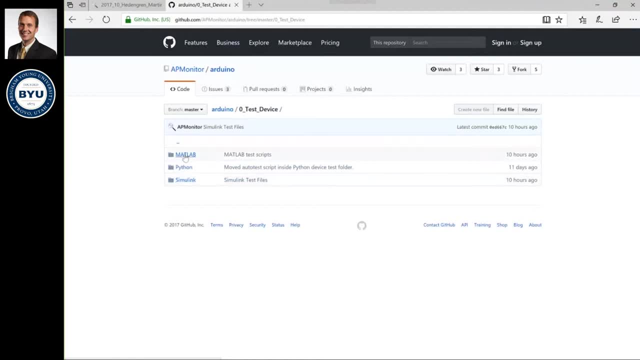 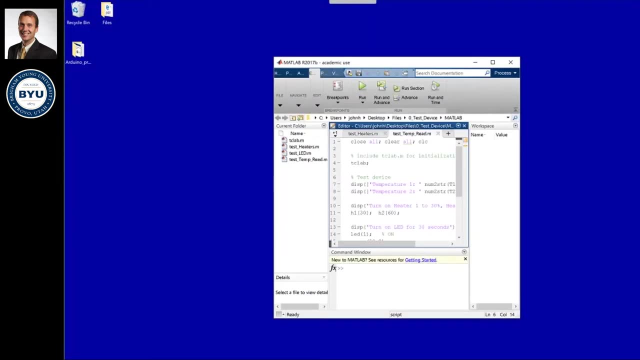 Python and Simulink test files, And so the very first one is just to test that the LED is blinking, And so I'm just going to go ahead and do that. So I'm just going to, first of all, I'll just go ahead and do this all from the command line. 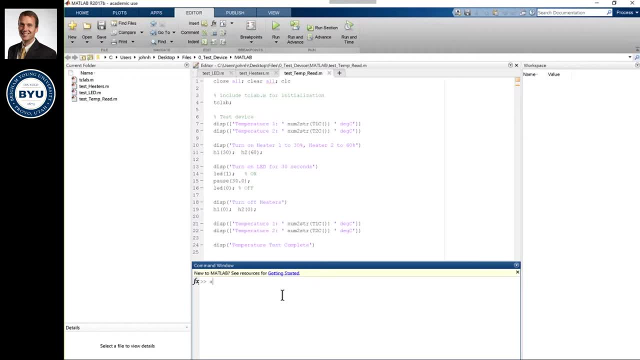 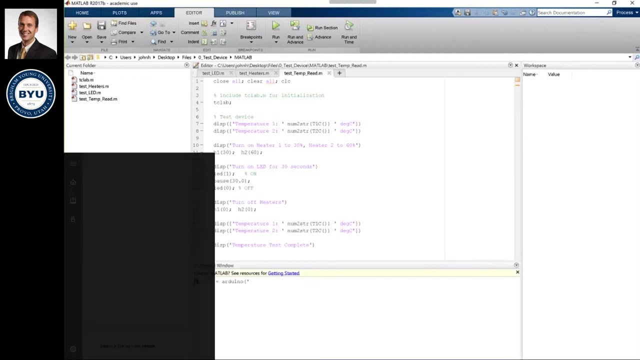 Let's see. I'll just do it down here. So when you connect an Arduino, you have to install the Arduino package first, And then, the very first time you connect, you have to tell it the port that it's on. So, for example, you would come to a device manager. 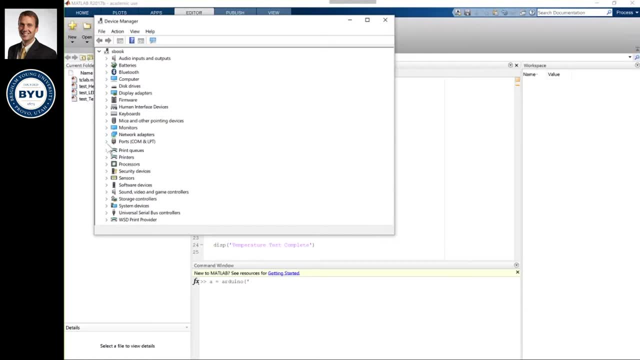 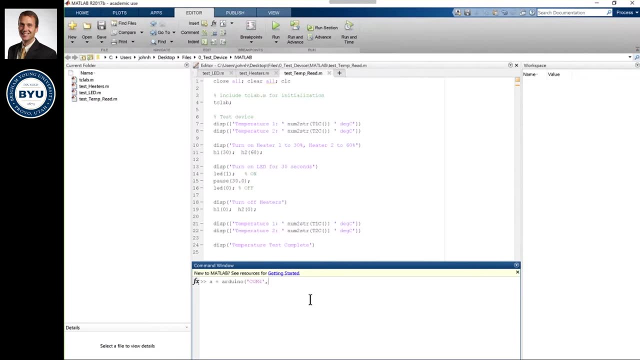 And figure out which port it's on. Okay, So I'm on COM4 right now And this extra configuration is only the very first time that you do it. Okay, So I'm going to connect to it And let me go ahead and turn on my webcam as well, just so you can see the. let's see if I can find that. 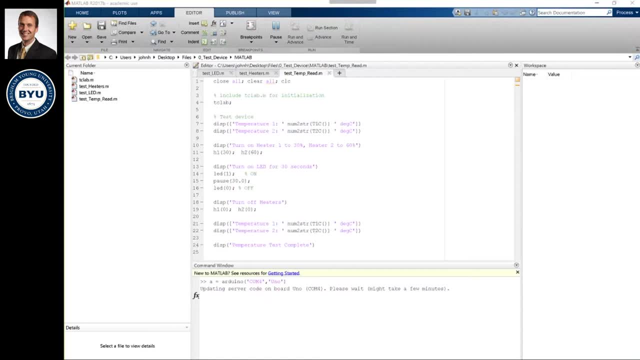 Okay, And I'm going to see if I can switch my camera view to the back one so you can see that. Okay, You can see that it's connecting to the board right now And it's downloading all the code that will be needed on that board. 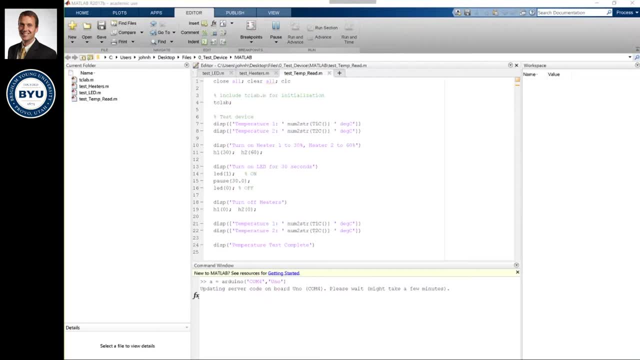 And see if I can select my camera here. I know I can select my back camera. Let me just try this. I'm going to put it on speaker phone just because I'm going to be using a couple of these, And okay, Can you still hear me? 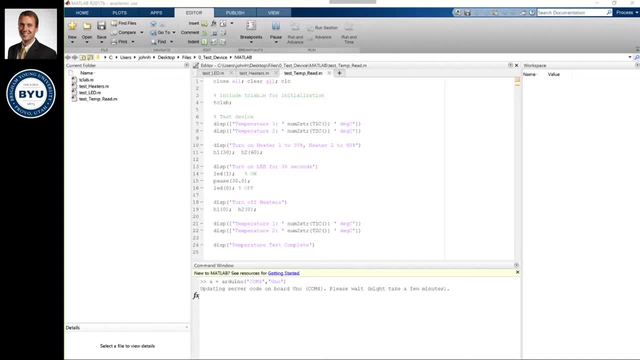 Yes, Okay, Great. So I'll just bring it to the front here, Okay, So I have this device right here, Here's the lab, And what we're going to do is just make the LED blink. So right now it's loaded in. 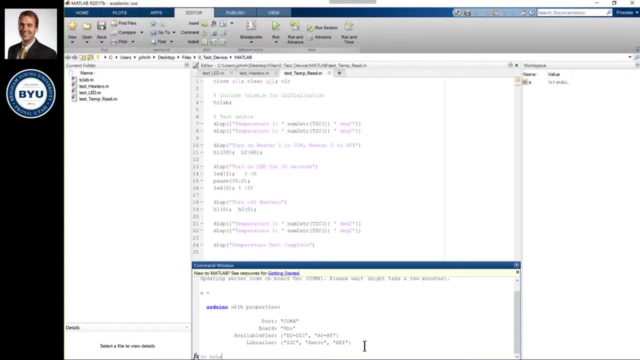 And then I've got a couple just Functions that I have set up in TC lab And what we'll do is go ahead and connect. We have COM4 that we connected to. Oh, I already was connected to Arduino, So I tried to. 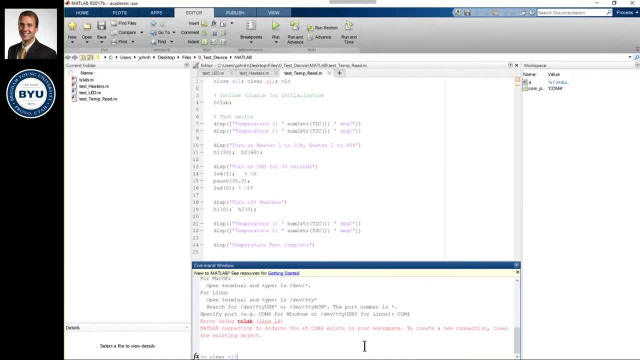 Let me just go ahead and clear it all And I'll start that again. Okay, So I'll just do TC lab And then it's going to connect to the Arduino And then, if I want to turn on the LED, I would just do LED 1.. 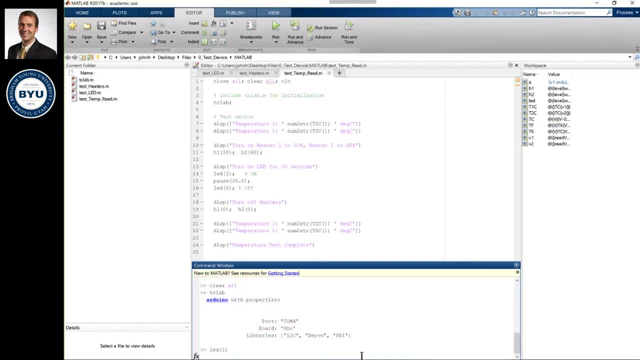 For example: Okay, So here it goes, And the LED turned on, And if I want to turn it off, I'll do LED 0. Now the other thing I can do is go ahead and turn on the heater. I'll turn on heater 1.. 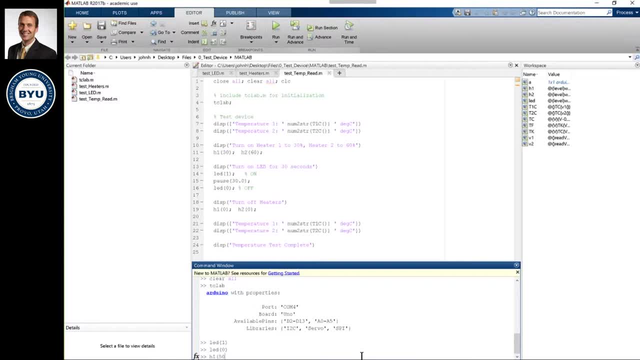 I'm just kind of typing with one hand here And I'll set it to 50.. Okay, So the heater 1 is on to 50% right now, And then I also want to do T1C, Get the temperature, the current temperature. 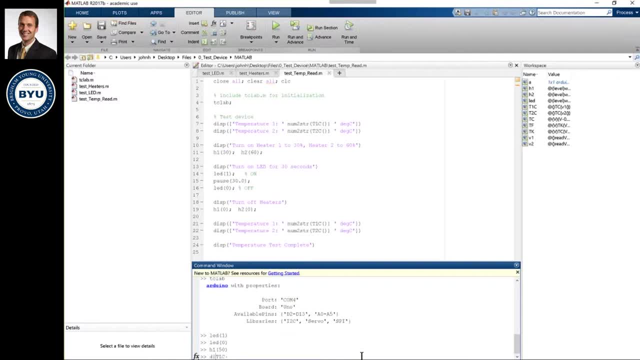 And I'll go ahead and just display that. It's a little bit hard to type with one hand, But there it goes. There's the temperature in degrees C, And if I keep hitting up I can see that the temperature is going up. 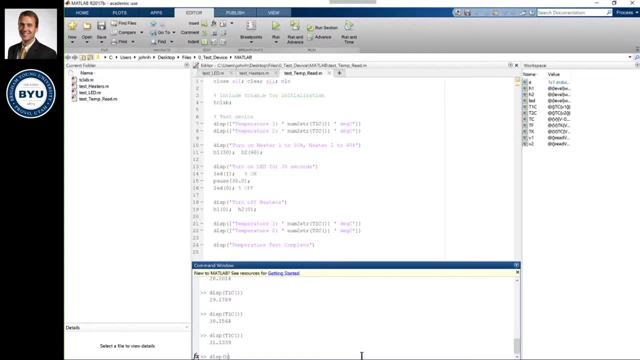 Okay, And then I'll go ahead and set the heater 1 to off or 0.. Display heater 1.. I didn't need to do display there. Okay, There we go. So that's just kind of the basics on how to control the heaters and the LED. 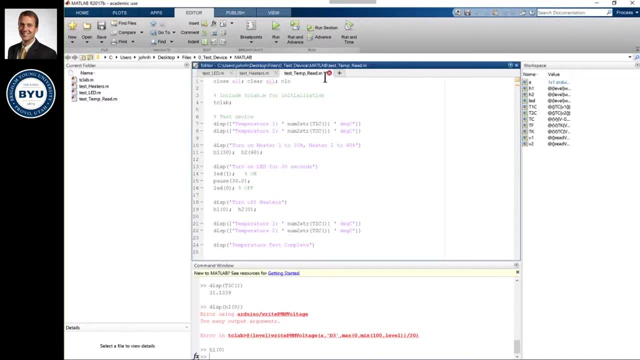 And read the temperatures. And then there's a couple other scripts there as well. I'll go ahead and run this one. This one is the test of the heaters And it's just a basic step response, And so it just runs through. 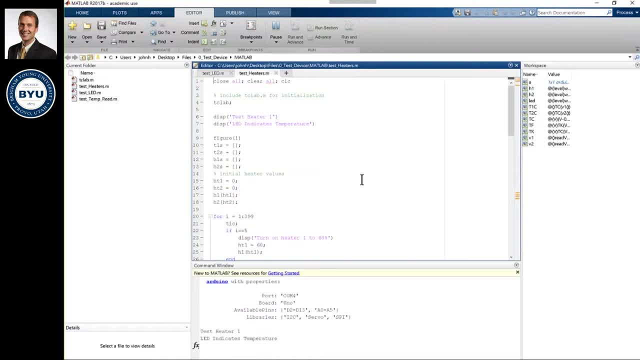 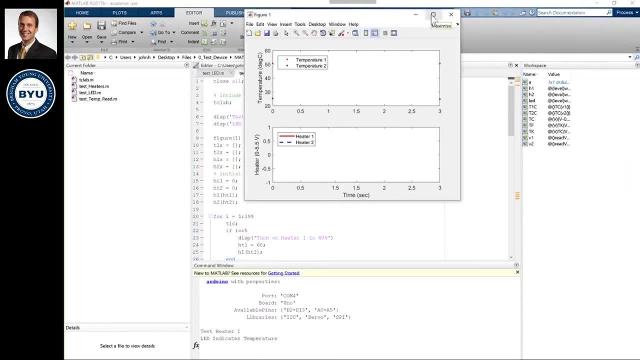 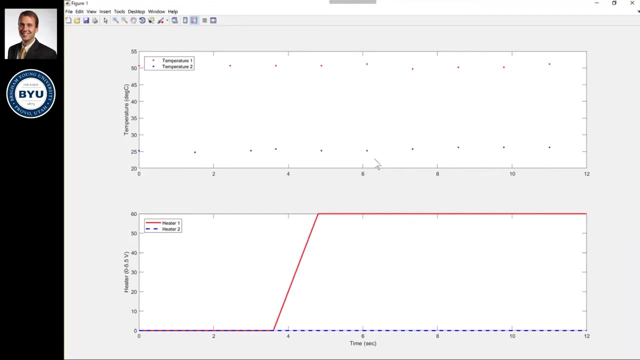 And with the script and a for loop it's going to, you know, go through and do this step response. So students might do this as maybe a first exercise. They might come into the lab and step one of the heaters up And then watch the temperature response. 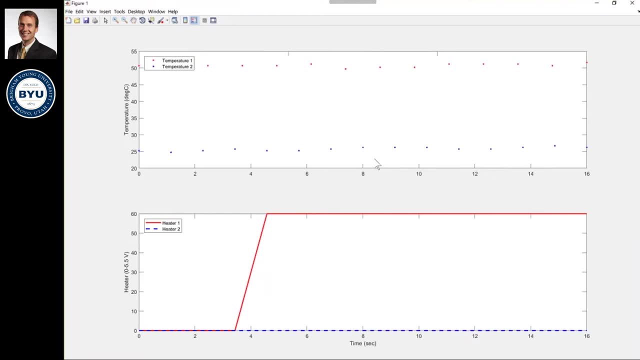 And you can see that I already had the heater on for a little bit And so the temperature increased. Okay, And then you can just watch the temperature increase And you know, students can collect data, save that data to a text file. do some modeling of that? 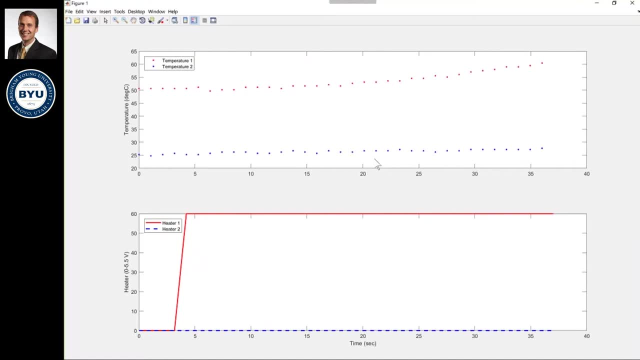 Most times we're just going to do single input, single output for introductory exercises, But there's also the opportunity to do multiple input, multiple output for that. Okay, So you can see the temperature rising. You know, in class you can have do things like change the heat transfer coefficient, maybe by setting a fan on it or blowing on it. 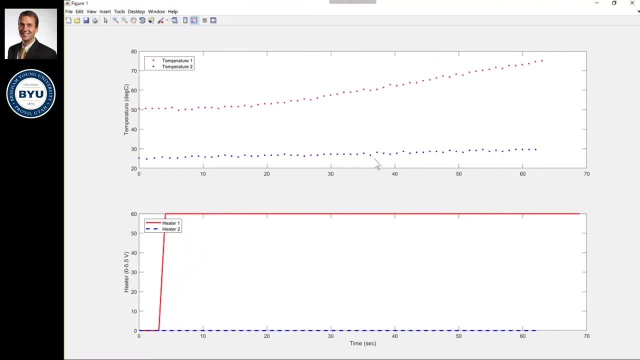 There's some other things you can do to, you know, partially insulate it and see how the heat transfer coefficient changes. So just understanding the dynamics of the system And seeing the real data streaming out, I think is valuable for students to experience. 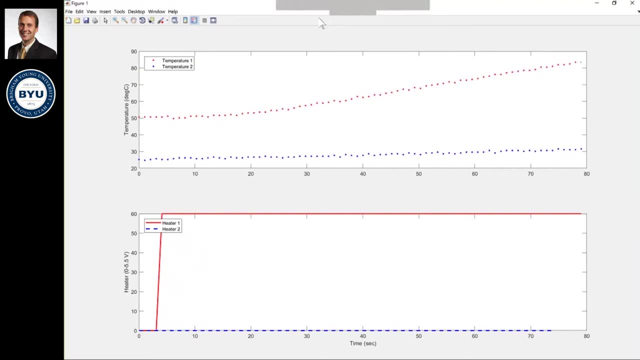 Okay, So there is the heater. Okay, So what I'm going to do now is that one is getting a little bit hot. I actually have a 9-volt in there right now, a 9-volt power supply, And so, just for safety considerations, we've actually gone back to using just a 5-volt. 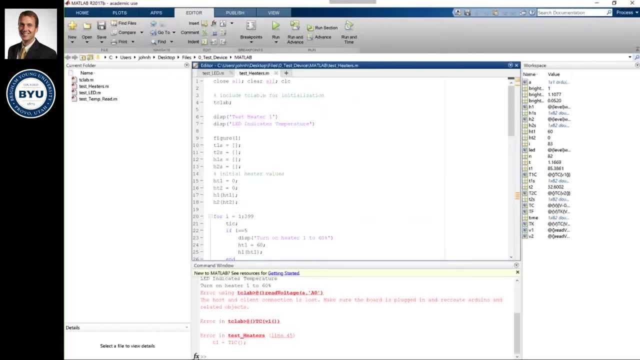 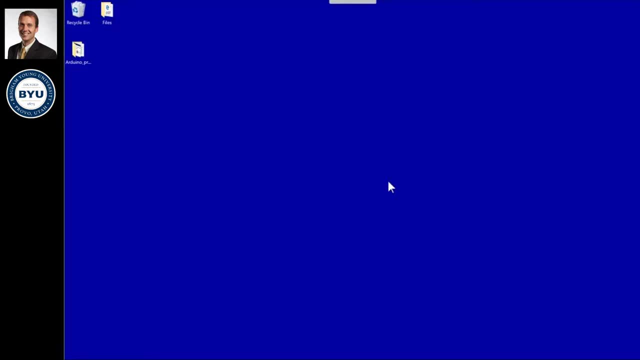 So it won't get as hot for the students. Okay, So I just went ahead and disconnected that. I just want to show briefly the MATLAB as well. We showed MATLAB. I'll show the Simulink as well on this. So these are the files that are available from GitHub. 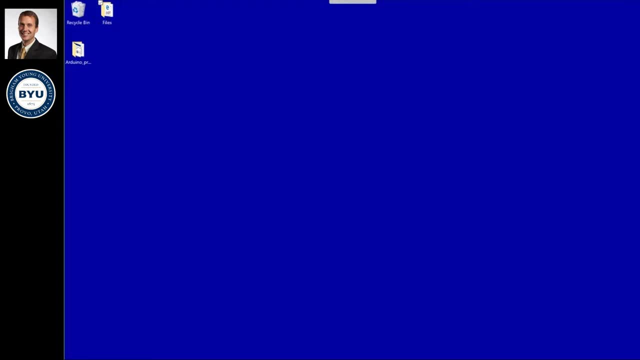 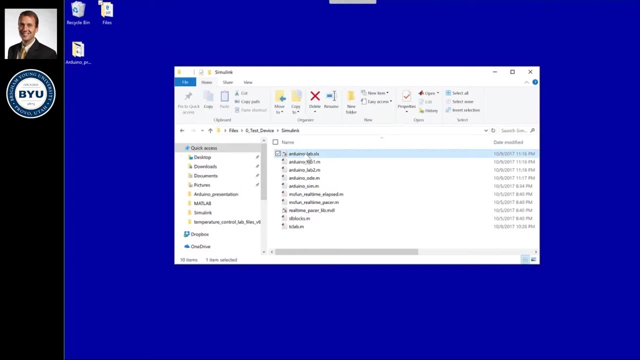 And so if you come into those files, you'll see a Simulink, And here is the Arduino lab for Simulink. It's just a block that you can do. It's a block that you can drag into a Simulink model and then be able to use the lab. 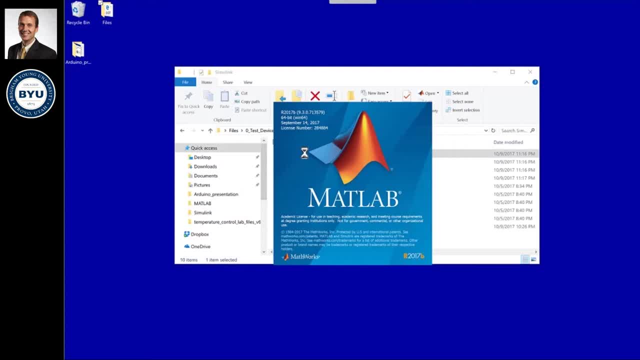 Okay, Now I had to identify the port. you know the COM4.. You only ever have to do that the very first time you use the lab, And then it has all of the device drivers that are on the Arduino lab. So when students use it, that's just going to be an issue for the very first time. 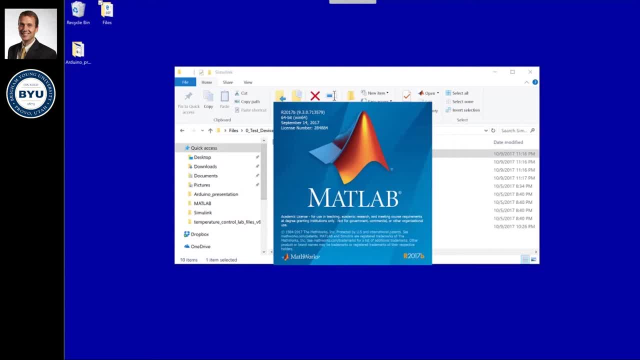 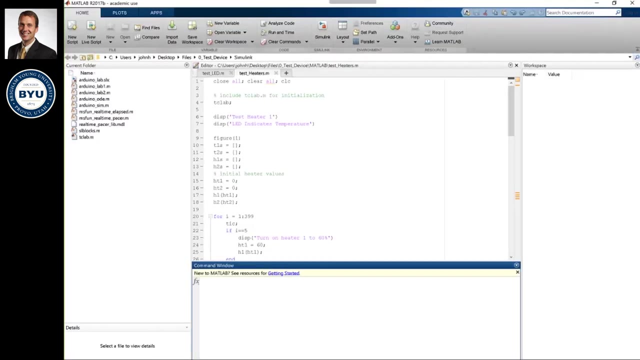 So I'm going to go ahead and just Okay. So let me, Simulink is going to come up. I have the 2017B- you know the latest version of MATLAB- loaded And we'll see a Simulink model come up. 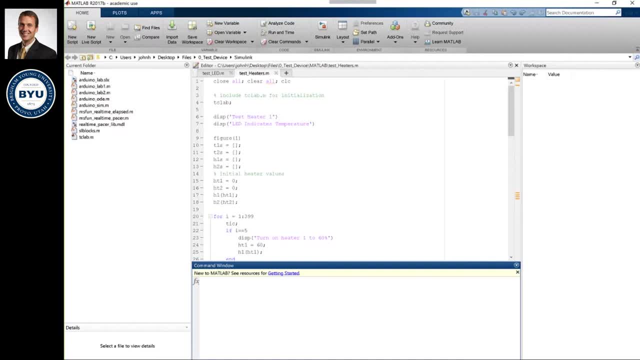 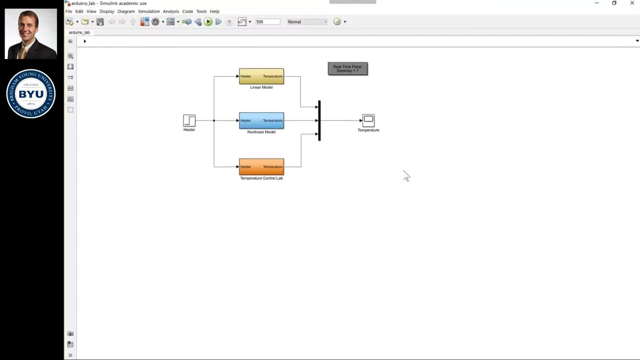 And then we'll be able to start this one. Okay, And then Okay, All right, Okay, And just as this is loading, I'll also mention I've got you know instructions for all these. I'll have videos set up to kind of step-by-step walk students through how to use this. 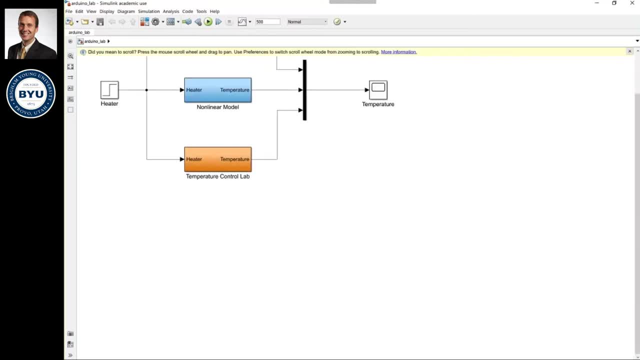 Okay, So this is a Simulink model that I have for the lab. One of the things that we have students do is compare a linear model, a nonlinear model, and then they also have the test model, And then they also have the temperature control lab. 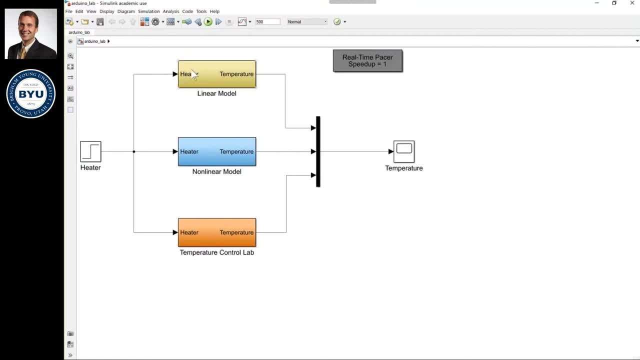 And so for each of these, the input is going to be the heater coming in and then the output from that block is going to be the temperature response. And for the linear model, if you just select that, it's a first-order plus dead time model. 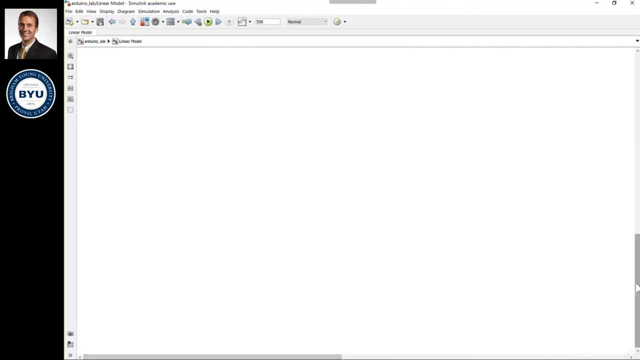 I'm going to make that just a little bit bigger so you can see it, Okay. So there's the model, Just a linear model with a gain and a time control, Okay, And a time constant and a little bit of delay. You also have the initial temperature and then those will – it produces that output. 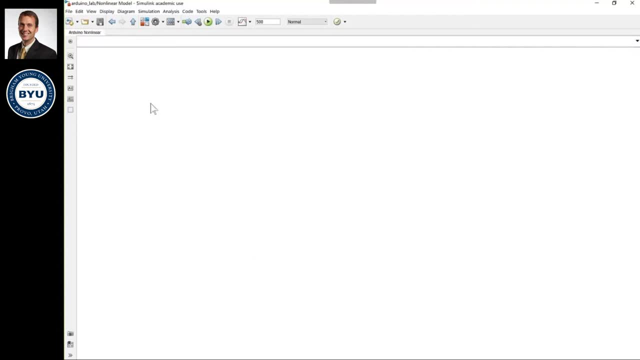 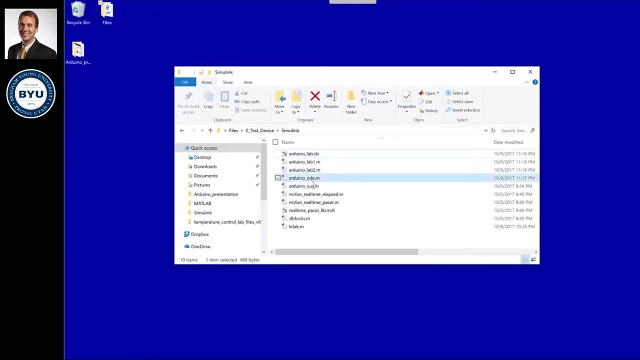 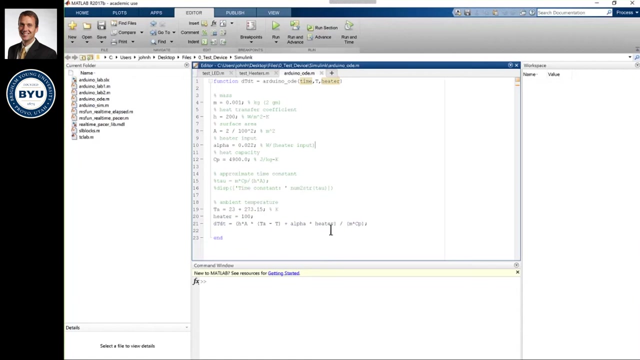 Okay, We also have the nonlinear model there. I just gave this as a resource with an ODE through Arduino Sim, So students will take that and then modify the fundamental model more fundamental model that is located here in Arduino Sim. Okay, And then they can add things like you know, answer questions like: well, do I think you know convection or conduction? 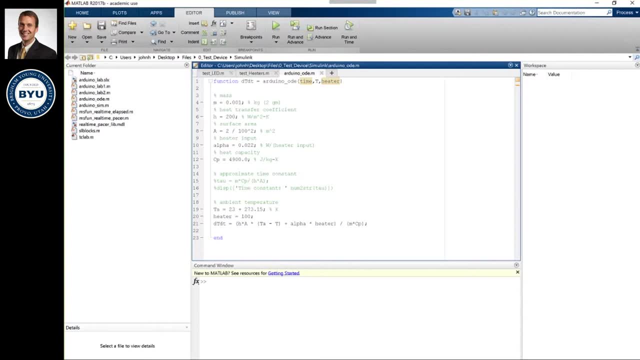 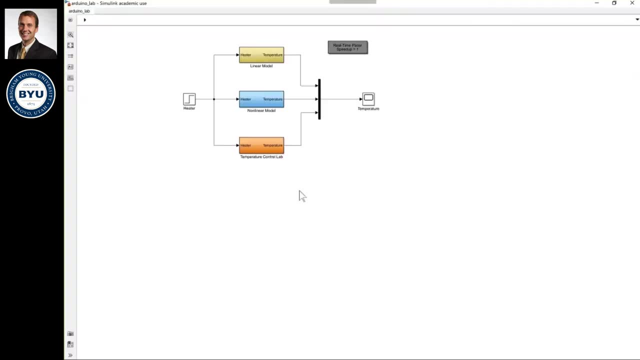 or radiation is going to be most significant, And they can model that and then try to answer some of those questions. Okay, So let me bring this one back up. Okay, So I'll go ahead and start this one. Let's just go for 270.. 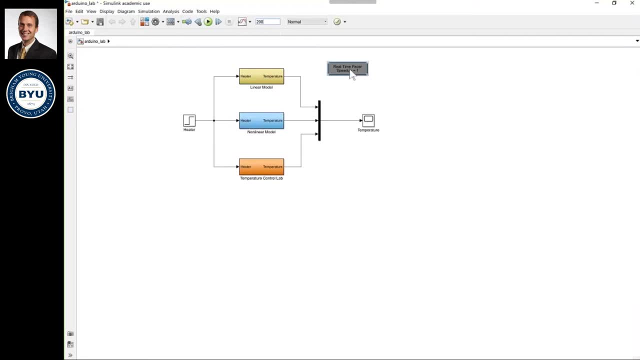 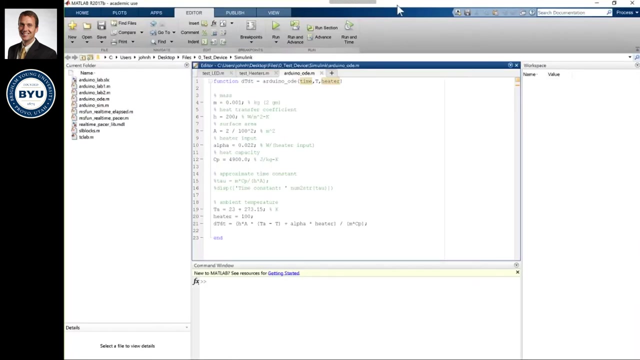 Okay, 200 seconds. And then I have this real-time pacer here to make sure that the simulation time matches the clock time. Okay, So let's see if this thing has any warning messages. for us, It looks like it's okay. 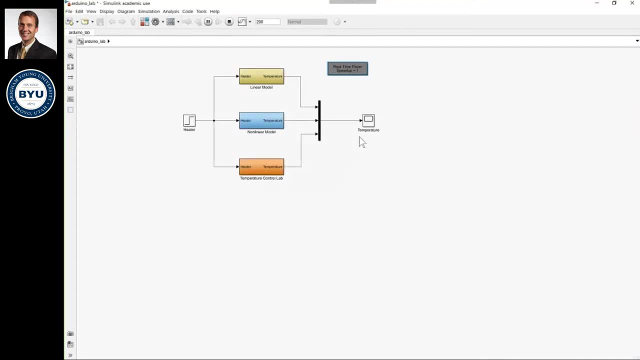 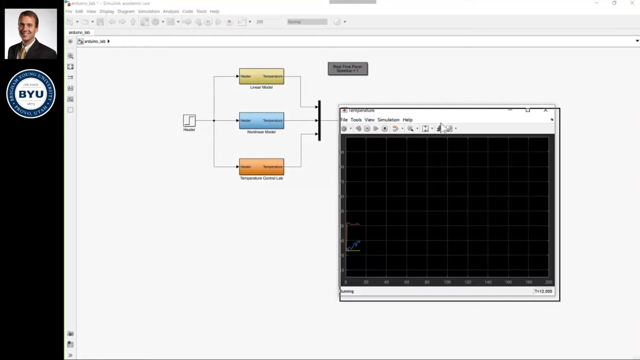 And it's compiling And then it starts to simulate And then we can see the, you know, opening up this temperature response, And this would be one of the very first things that students would do as part of the lab is try to model it. 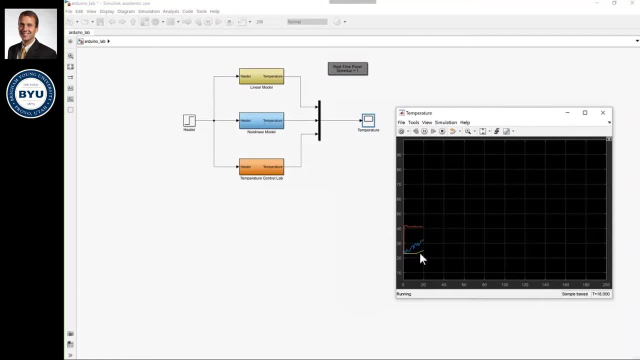 Okay, So I added some noise to the nonlinear model, But you can see the linear model. We had a step change in the heater And you can see the three that are going to be tracking. And then, invariably, the students will get to this point and they'll be trying to model it and they'll see a difference between the predictions and the actual data. 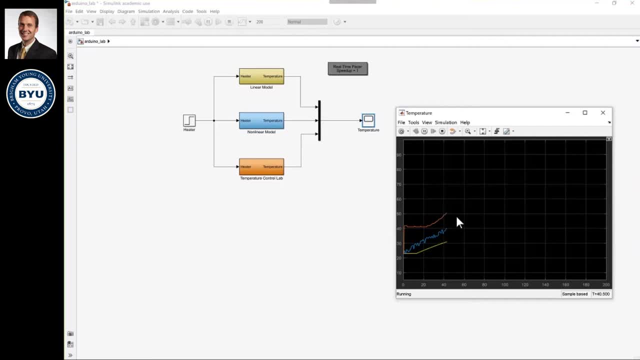 And then they'll, you know it will cause them to iterate many times, you know, to go back and revise the model and try to figure out what's not working. You know where is there a gap in understanding, Where are assumptions that may be incorrect in their models. 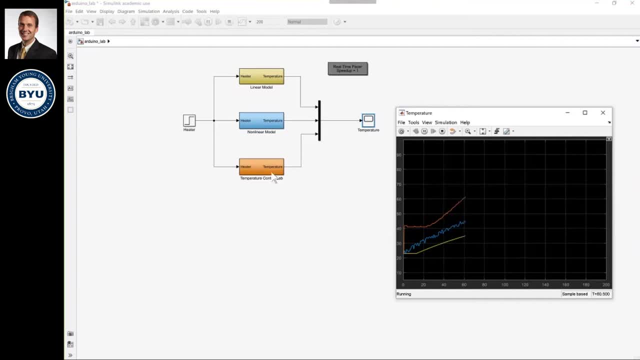 And so we have these three models represented by these three blocks, And this one is actually the physical device of the system. Okay, And so there's going to be students go through the exercise of doing some identification, either parameter identification through optimization or manually as well. 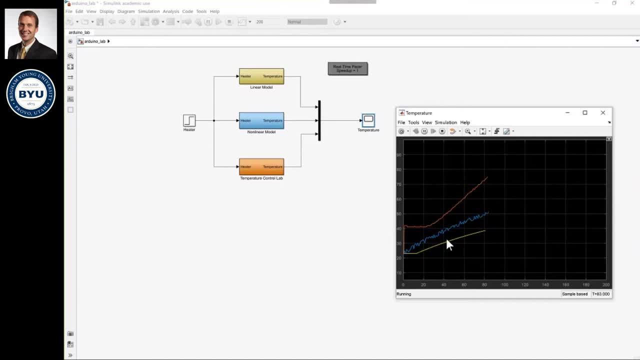 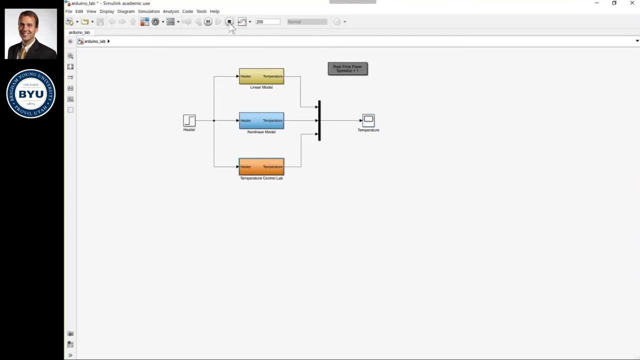 And they try to make these three match up best they can. Okay, So this block right here- I'll go ahead and just stop this- This block right here can be put into something like a PID, you know, controller with feedback control within Simulink. 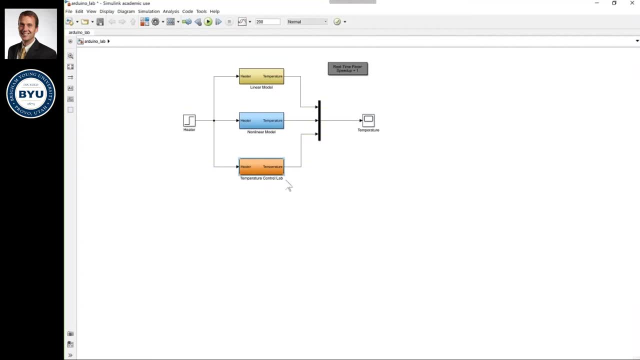 It basically just has the input heater and then the output temperature, And then students can drag that around and make different types of configurations that they'd like. Okay, And that is all from the Simulink side. We'll go ahead and turn it over to Jeff now. 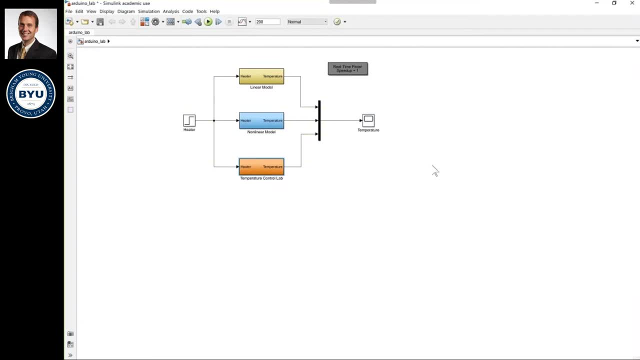 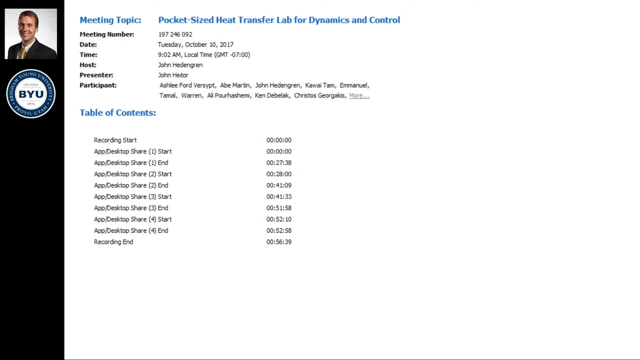 Jeff, do you want me to just have you share your screen? Yeah, If you could just share my screen, that would work best. Okay, You're the presenter now, So go ahead and Can you see my screen? okay, Not yet. 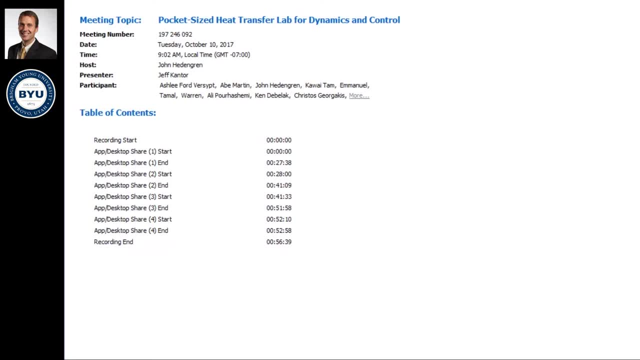 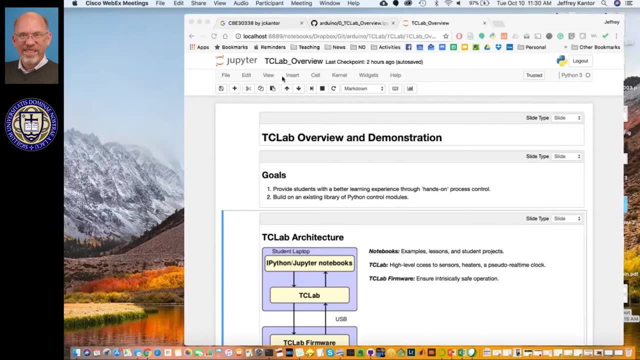 You may need to click share and then my desktop. Okay, Share my screen. Great, And are we going now? Yes, Okay, Great, Well, thanks, John. I'd just like to take a few minutes and I'll do a demonstration using some Python tools. 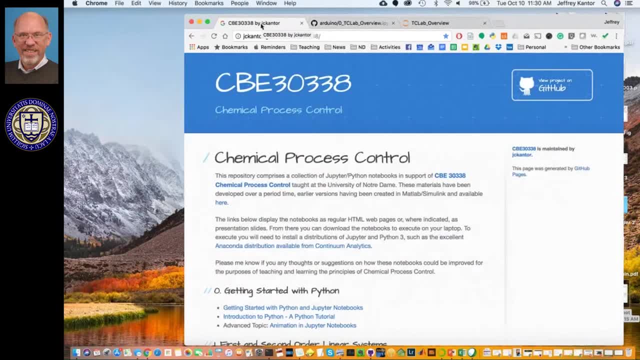 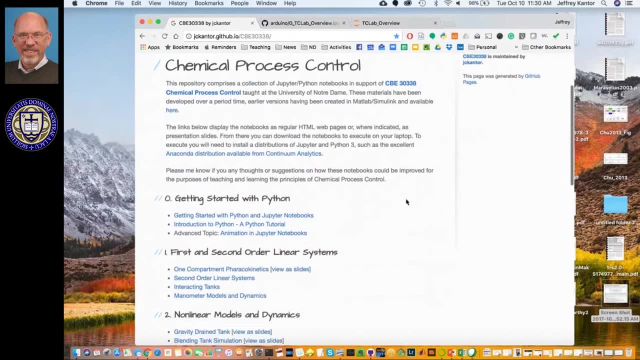 But by way of background I've been teaching the process control course for a number of years And in the last few years have developed a series of control of notebooks in Python that walk through the full curriculum, And so here I'm showing from my GitHub account. 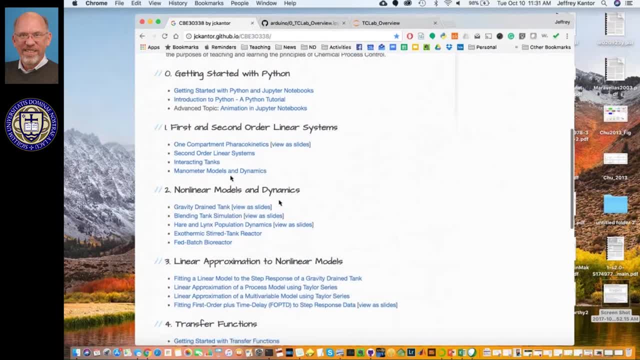 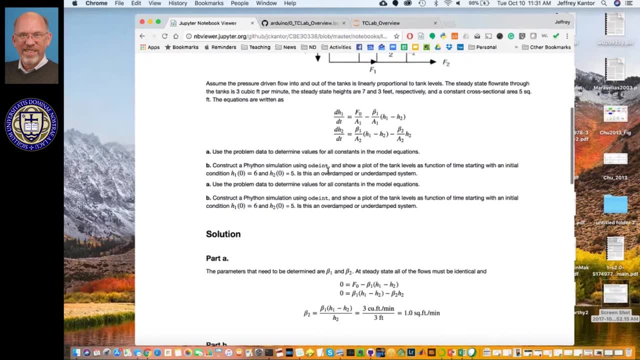 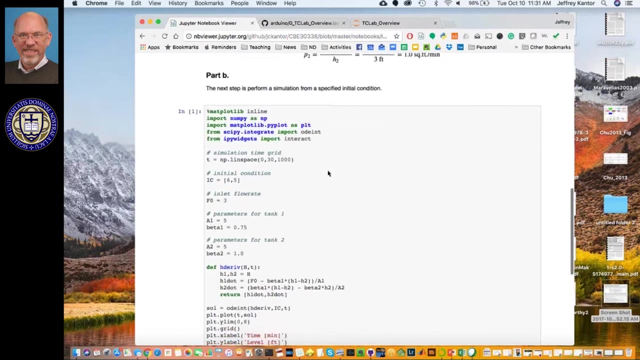 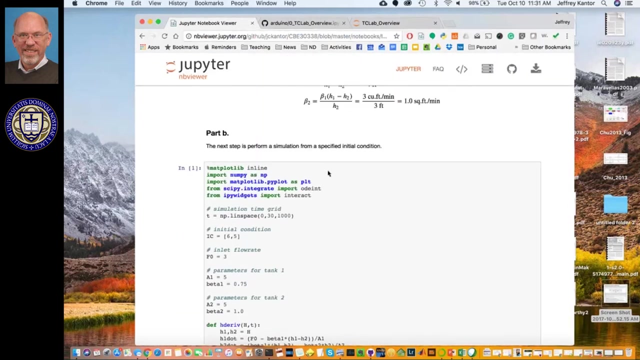 Some of the notebooks that I've developed over those years. For example, here's a module on interacting tanks, And this is a lesson that includes some basic modeling, In this case, a simulation that's built in Python. simulation results And I've been able to build up pretty much a full curriculum using tools open source. 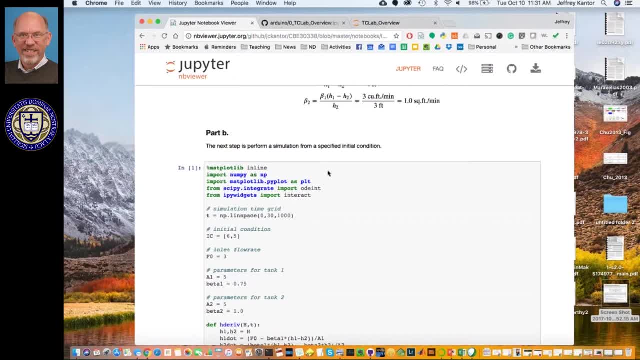 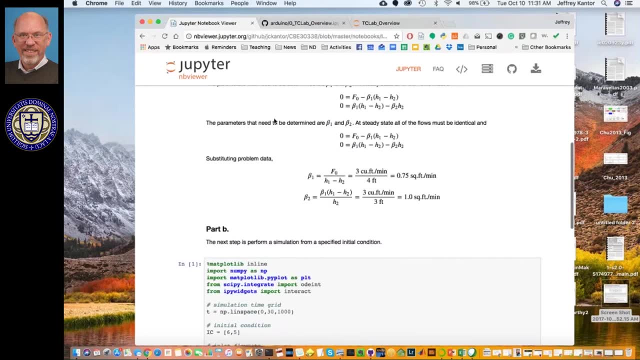 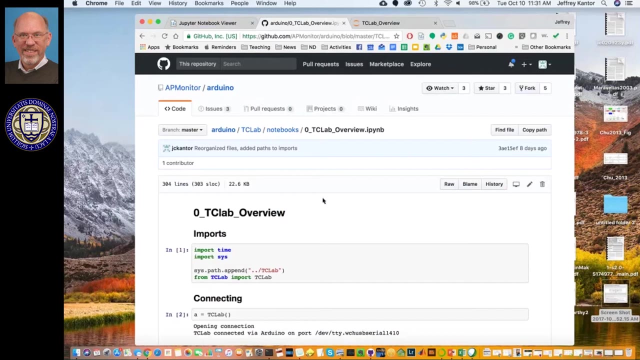 tools And, in particular, the control systems toolbox that Richard Murray has developed at Caltech. So my starting point is this course that I've developed and will continue to teach, based in Python, And so, when it comes to this lab device, I'm very interested in providing a hands-on experience for our students. 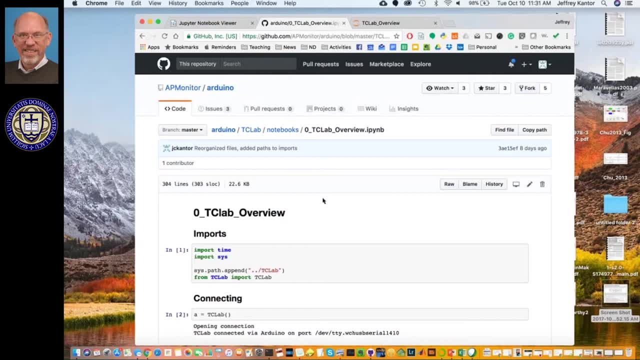 We have a mandate from the university to try to do a better job in making a smaller class environment for our students. It's a challenge for us When we have just a few faculty teaching so many chemical engineering students. So my plan for the spring is to teach two traditional large section lectures a week. 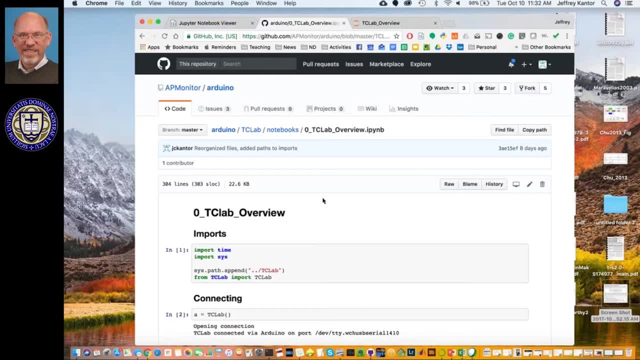 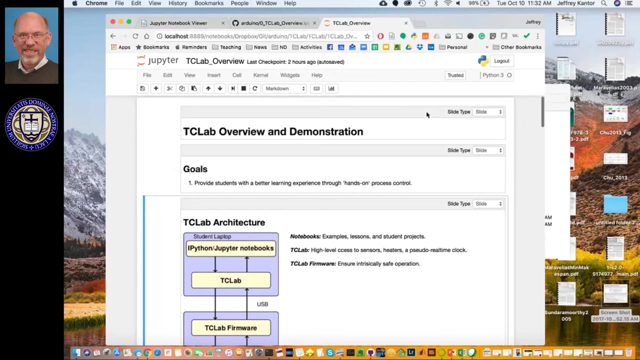 And introduce a new Friday afternoon lab sections where the class will be broken down into smaller sections And then students would work in groups of two using the temperature control lab. So what I'm envisioning is a weekly lab exposure to this device. So let me go to a notebook that kind of gives some a little bit more information about this. 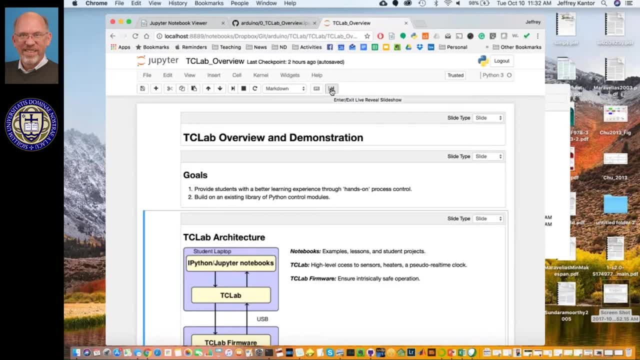 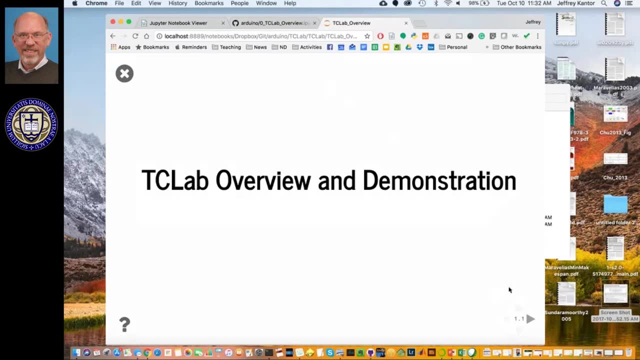 This is a Jupyter notebook, And one of the features that Jupyter notebooks have is the ability to present slides, So if this is working right, you should see a slide appearing on your screen. Is that what you see? Yeah, it looks great. 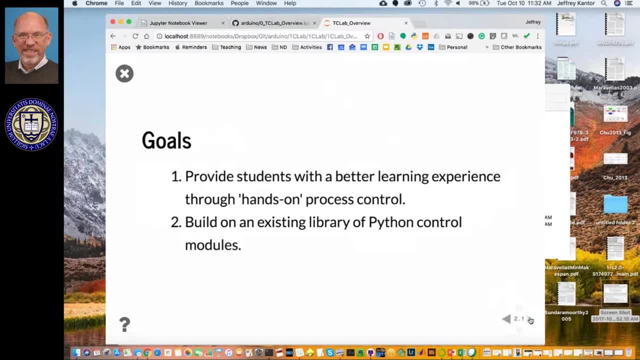 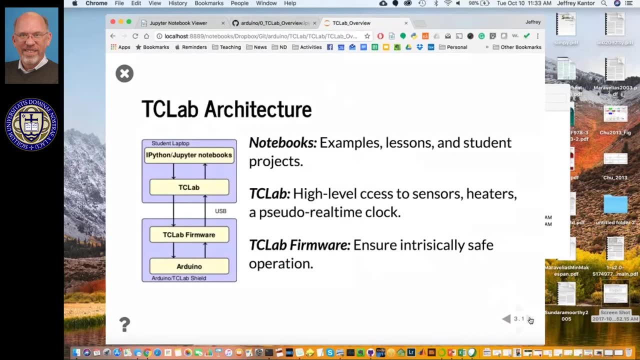 Okay, great, This is a live notebook, And so I'll be able to do the demonstrations from here. I've already mentioned the goals, so I'll just move on. One of the nice things about this device that John and the students have developed is that it's totally adaptable. 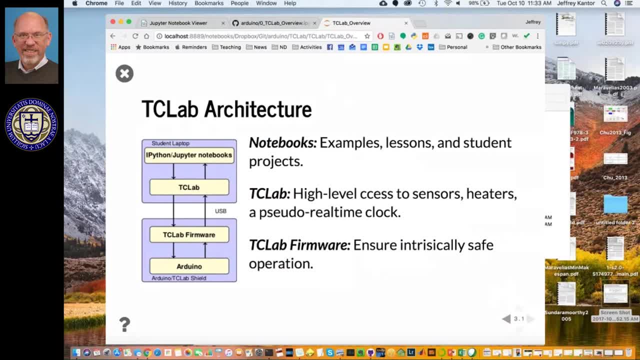 And so over the last few weeks, since I got my hands on the demonstration version, a development version of this thing, I've developed kind of a three-level hierarchy for this that I intend to use going forward, A little bit different from what John and the students have done. 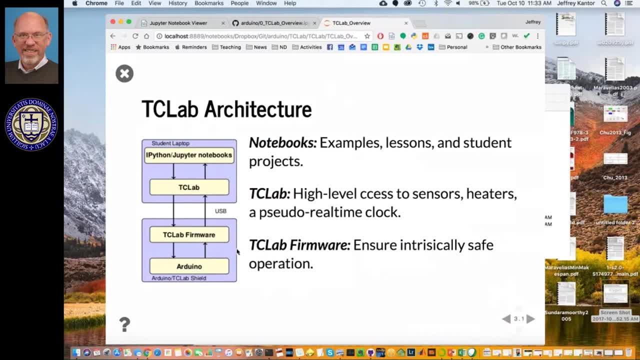 I have a little bit different philosophy than this, And what I'm using at the lowest level on the firmware side is some custom firmware intended to provide some safety features. In this case I'm using the LED is totally in the control of the firmware. 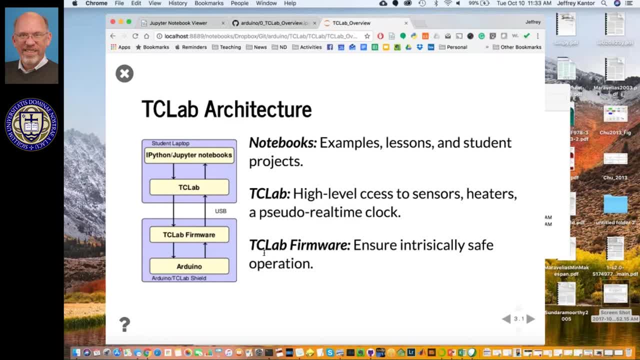 The students do not have the ability to use the LED because I'm using it to provide a status report on the condition of the hardware. For example, if the heaters are on, then the LED is bright. If the heaters have reached a temperature where you might burn a finger, the LED blinks. 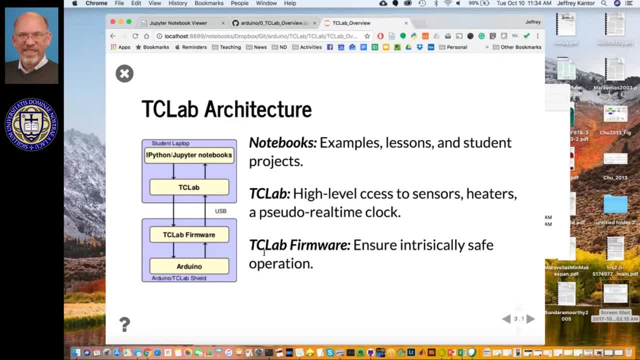 Then there's a sleep status and so forth. So the idea is to provide a little bit more of a distance from the student to the firmware. Then what appears on the student laptop is a module called TC Lab that provides a high-level access to the sensors and heaters and kind of a pseudo real-time clock. 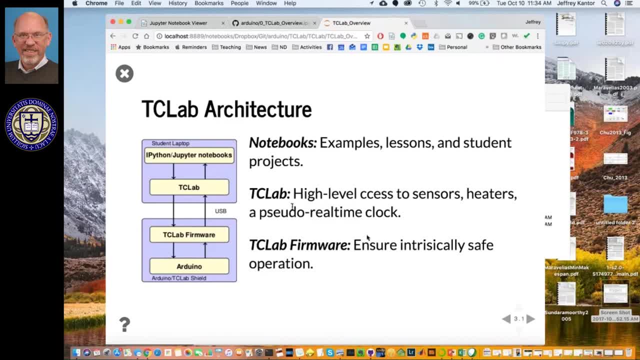 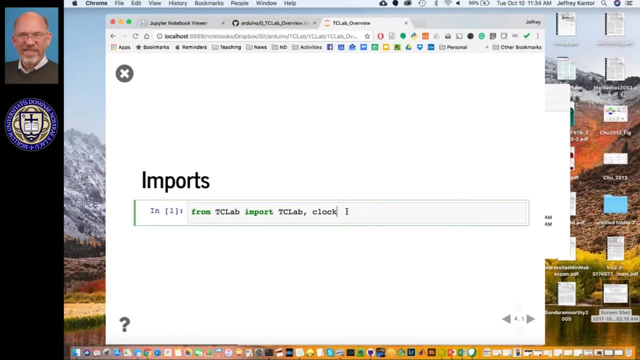 And then at the highest level, notebooks, And what you're looking at is an example of a notebook. Now I'll just kind of walk through a simple demonstration. So here would be the first line in any student code, And I'll run this now. 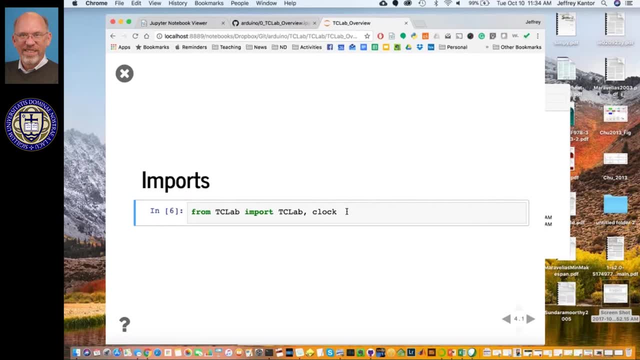 And what this is doing is it's loading up from the library the TC Lab module and the clock module. Now I just plugged in my Arduino device, I just plugged in the TC Lab And let's see here I now need to connect to it. 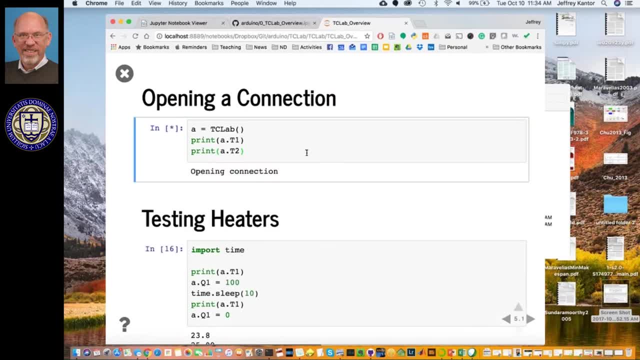 And so I'm going to connect to it with this command. And so what this is doing is it's using the TC Lab module to create an instance in Python, And then I'm using that instance to access the temperature T1 and temperature T2 and just printing them. 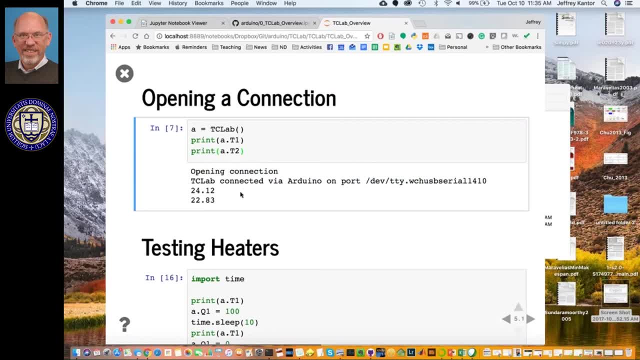 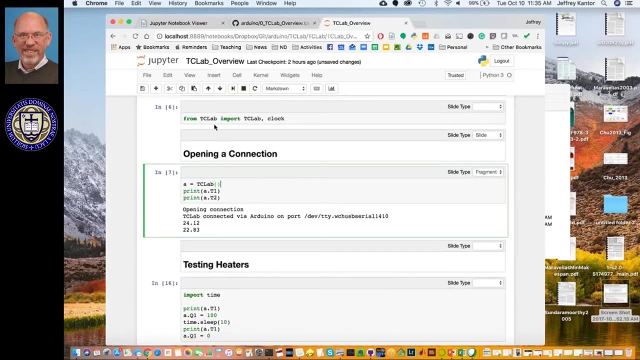 And so the current temperatures of the two sensors are 24 and 22 degrees To test the heaters, let me just add. let me go back to the notebook. You can still read this just fine. I'm going to add a cell here and then just show you how this works in real time. 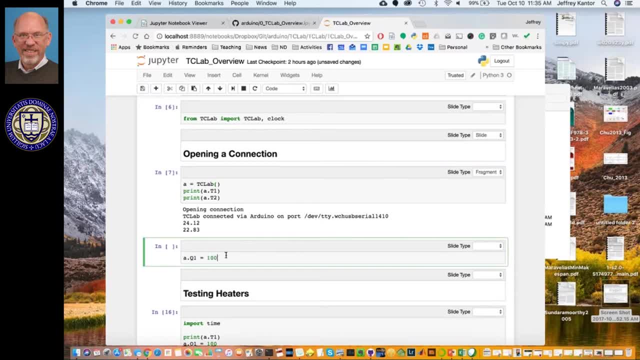 So if, for example, I want to turn a heater on, I can turn it on. with a setting of 100 millivolts, It's on. now I can add a cell. I can now watch the temperature grow. So let's see what's happening to temperature T1.. 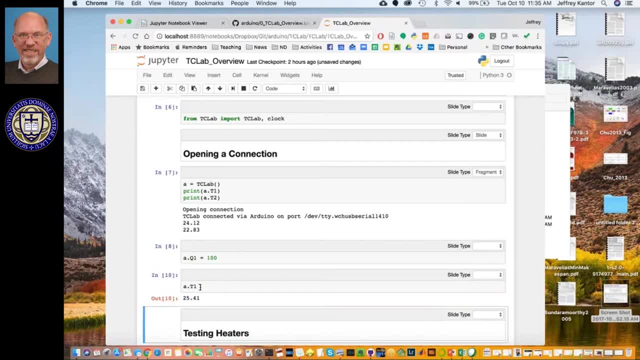 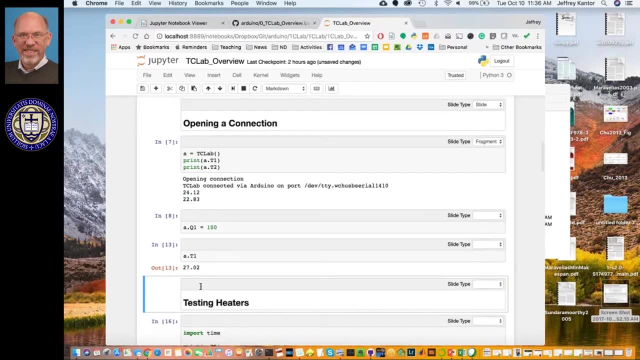 It's getting larger. I'll run that cell again. I see it's going up, going up slowly. Now it's going up a little faster So you can watch the temperature rise. You can see that I'm accessing both the heaters and the sensors as if they were just variables within the Python environment. 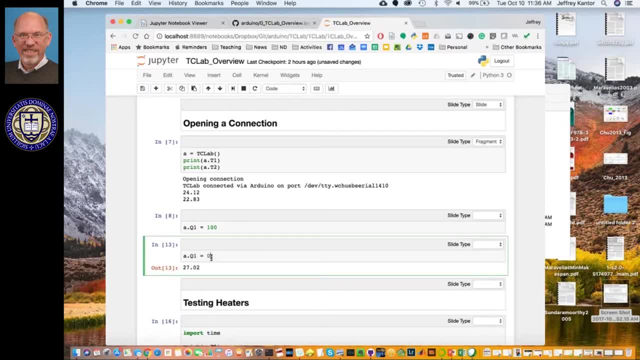 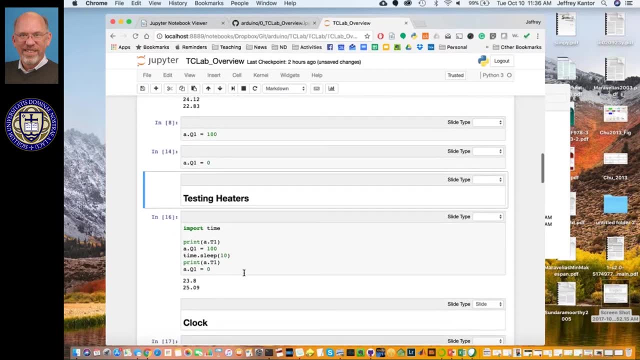 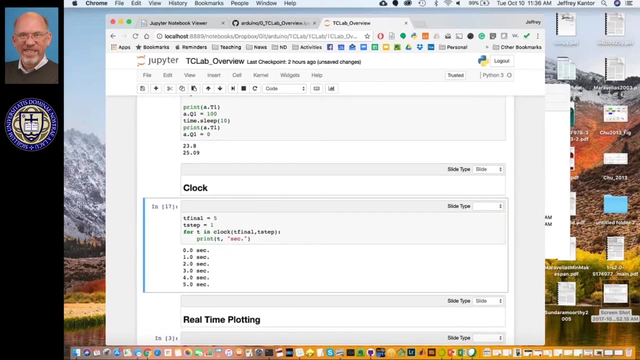 Now I'll just turn off the heater by just turning it to zero. So that's the basic high-level interface to the T1.. That's the high-level interface to the sensors and the heaters on the board. Let me go down to this cell. 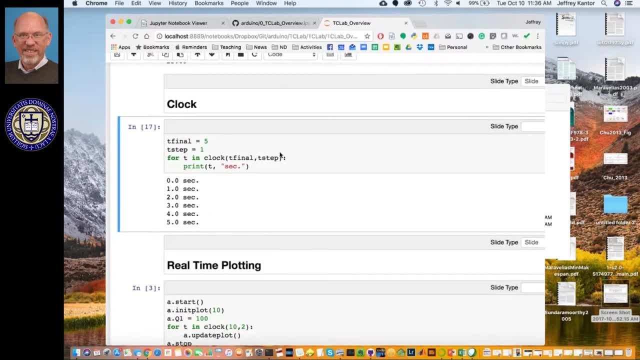 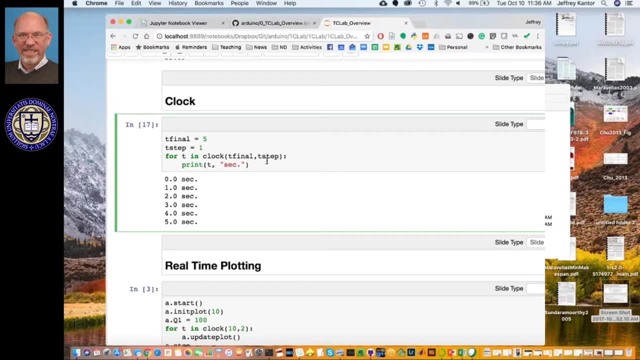 And here what I'm showing is a clock module, And this is a function that accepts as a first argument how long you want to run the clock and then the step size. I'm going to just run this for a few seconds, just to show you how this works. 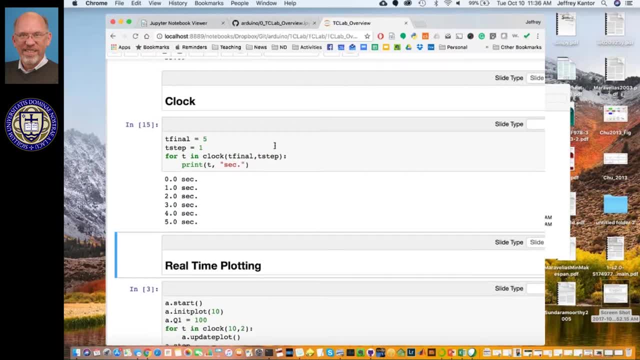 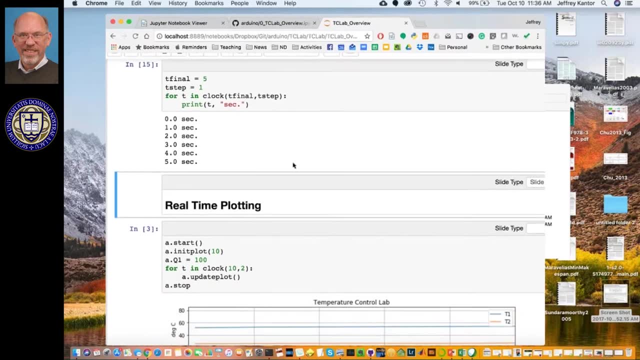 There's a pseudo real-time clock that's part of the module. It's not hard real-time. We get a dither of about a hundredth of a second or so. So it's plenty good for the kinds of experiments that we're doing. 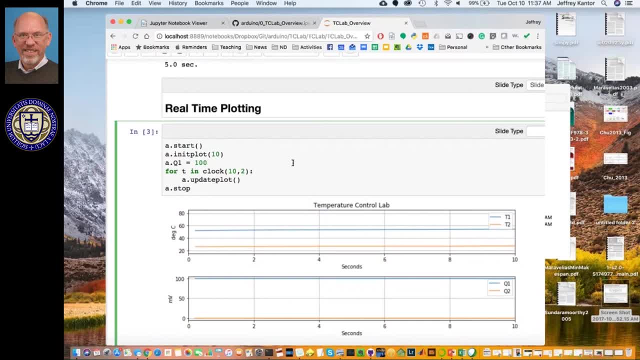 And then we have some real-time plotting within the Jupyter Notebook here. So the way this works is: the first command here restarts the Arduino interface. I set up the plot to plot for 10 seconds, Then I set the timer on to a level of 100.. 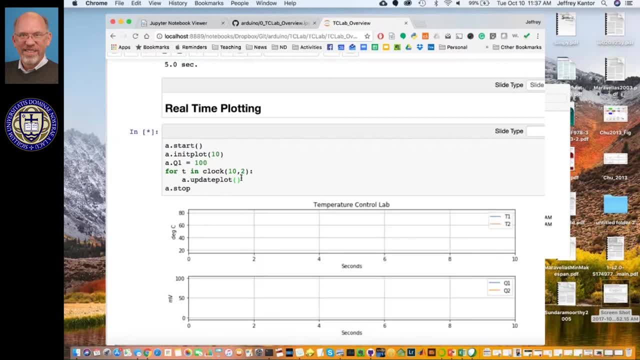 And then I just use the clock to sample the temperatures every two seconds and update the plot And you can see that moving along down below. So this sort of replicates what John was showing through his MATLAB and Simulink interfaces. So you can see what's going on there. 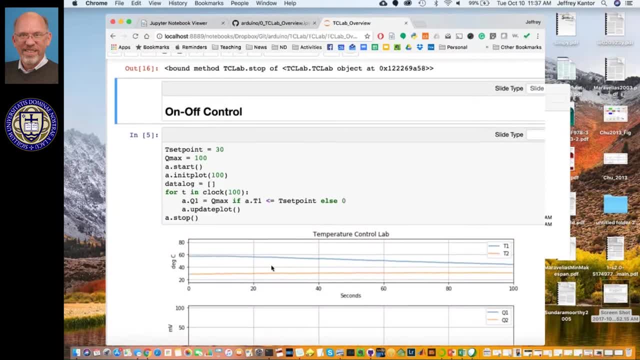 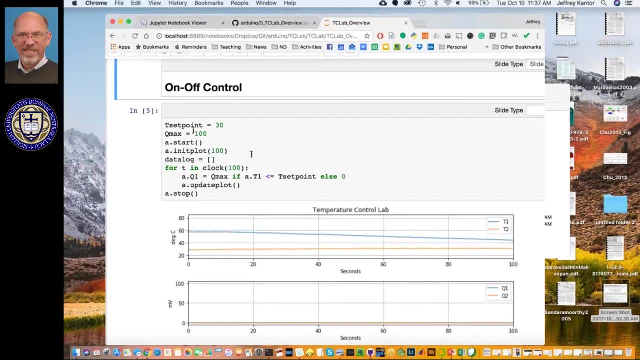 Now to demonstrate on-off control, for example. here's the cell that shows how a student could code an on-off relay-style controller for this. So what this is going to work is I've set a set point of. I'll change that to 40 degrees. 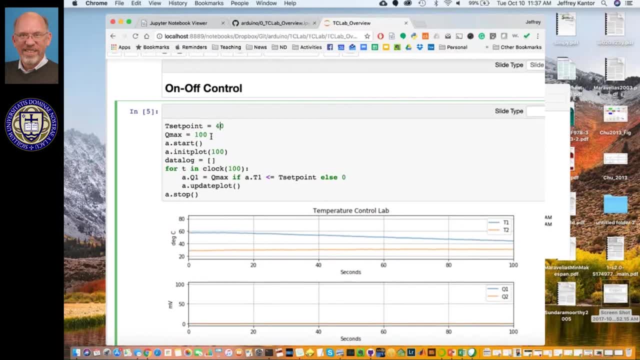 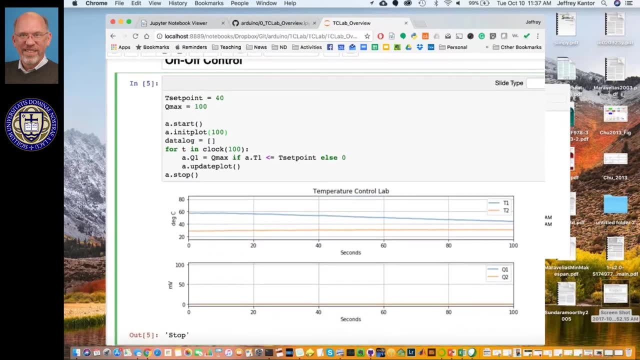 I'll set a maximum heater level of 100.. I'll start the device, I'll set up the plotting And I'll just drop that for now And we'll just run this Now each time through, so we'll get started. 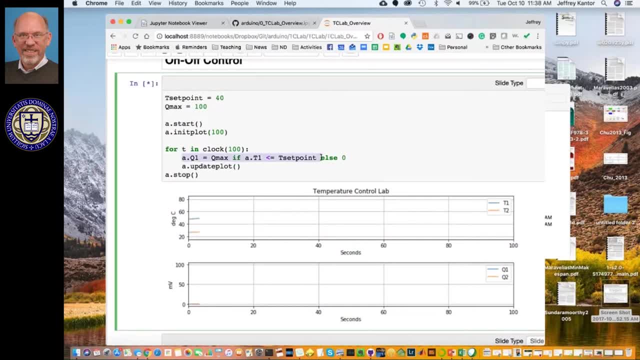 Now, as you look at the loop, each time through this first statement I'm highlighting right here is an on-off, And this is the controller. The heater is set to either Q max if the temperature is below the set point, Otherwise it's set to zero. 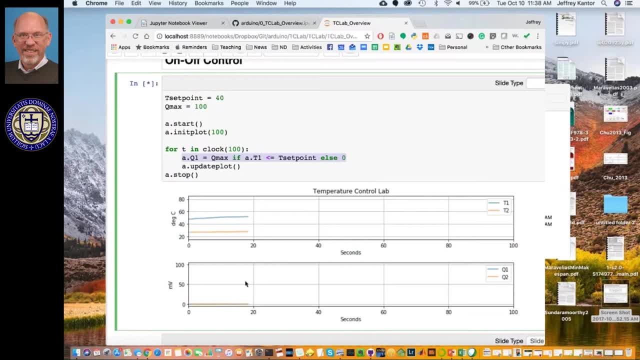 And we're going to see how well it works. Right now, the heater has been on a while and the temperature T1 is the blue line, So unfortunately, I think we're going to have to wait for it to cool off before we see the heater come on. 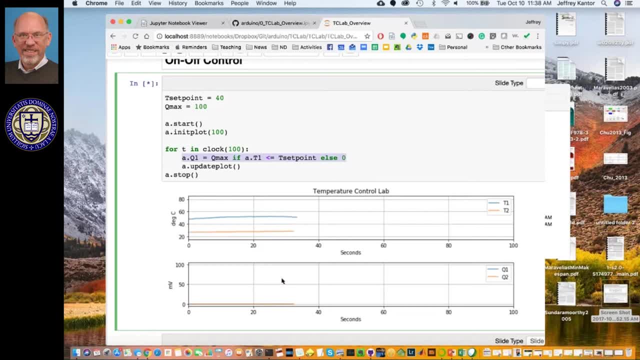 So I'm going to be blowing on it and putting my finger on it to try to cool it off as fast as I can. Cool it off as fast as I can for you. Ooh, that's a little hot. Okay, it's dropping now. 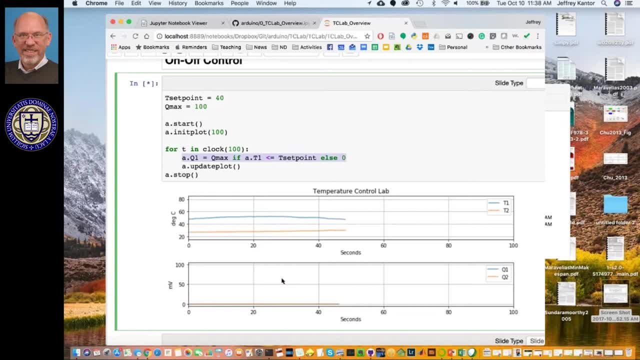 I'm going to blow a little bit more on it. Okay, we're getting it down, Okay, And so you can see the temperature T1 falling, And in a few seconds here we should see the controller turning on, Okay, Okay. so let's see here. 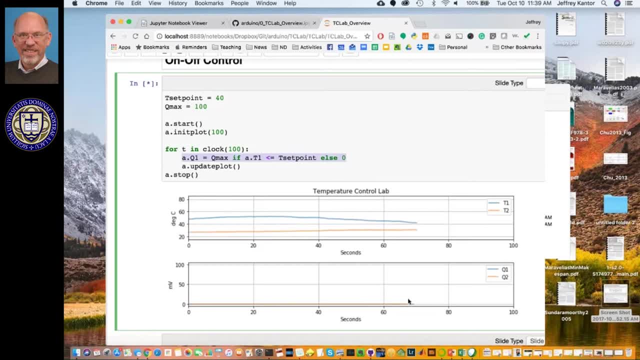 We're getting close, Okay, and then, in the nick of time, the heater just came on down below, And so you can see that the temperature is going to rise again And the heater will shut off here in a moment. Well, okay, that's the pitfalls of real-time demonstration. 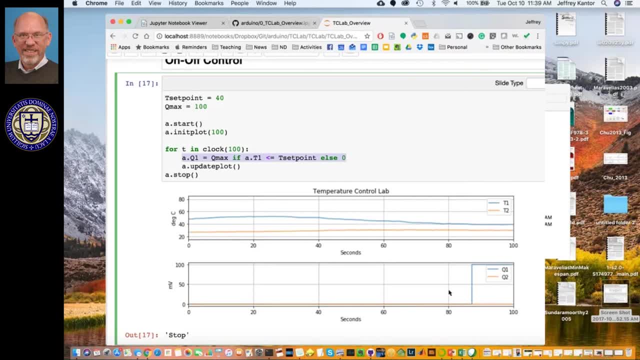 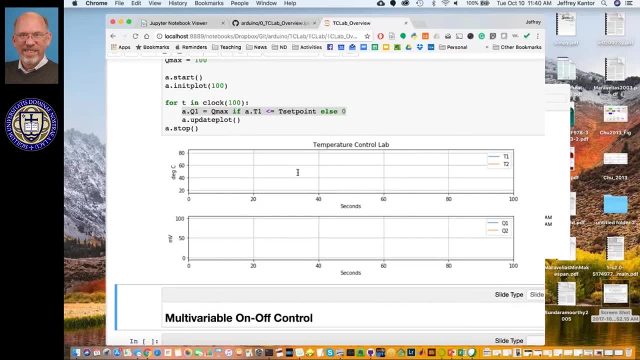 I was hoping to show you, hoping you would see the full cycling of the controller, turning both on and off, But I think this does demonstrate what's going on here. Now here's an example of a multivariable on-off control, where I'm setting an on-off controller on each of the heaters. 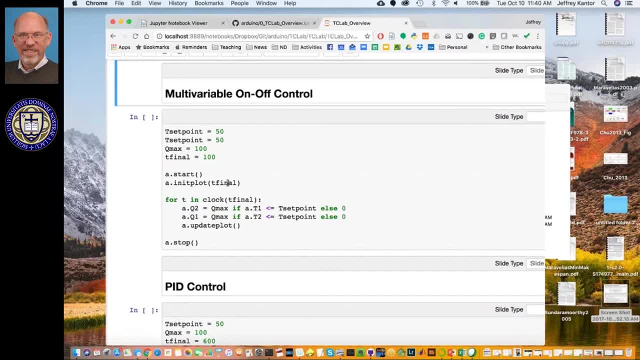 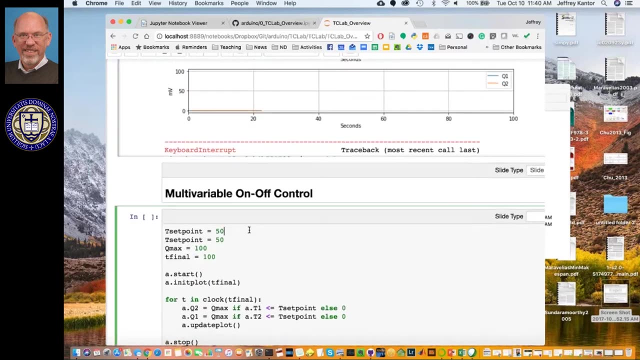 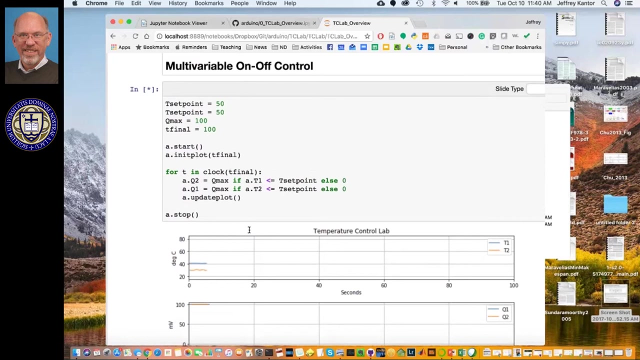 I've set the set points to 50.. Again, starting using a sort of real-time clock. This time it's the default one-second sampling, And I'm going to stop the clock above and then start the one down below. Okay, And so this time what we're doing is we have both heaters under on-off control. 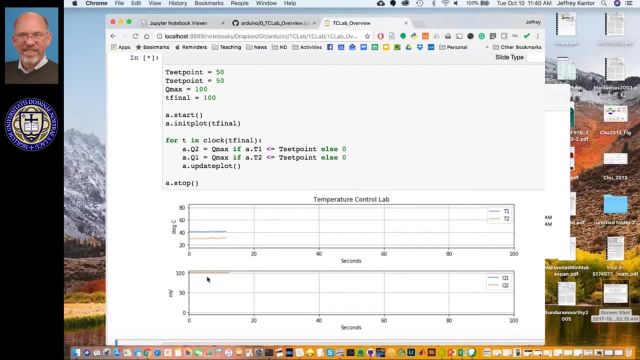 And on the lower panel you see that both heaters are at the bottom. These are the heaters that are at the level Q max And the temperature should be rising, And so we can see T1 should be getting close to a switch point now at a temperature of 50.. 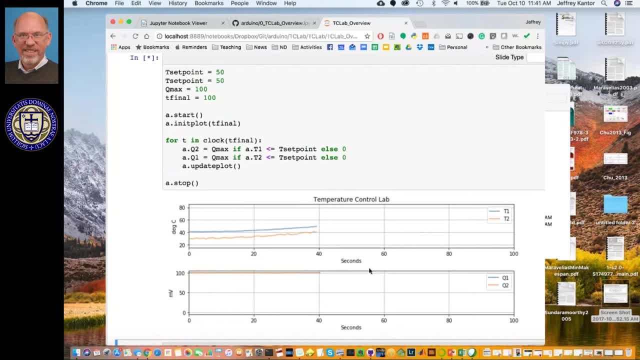 And so that controller should be turning off soon There. So Q2 has turned off. If we stop and think a moment about this. I have turned my controllers around, haven't I? So I've made a mistake in my control implementation, so I'll start this over. 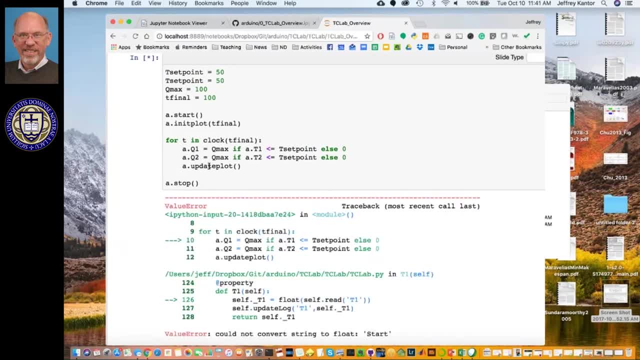 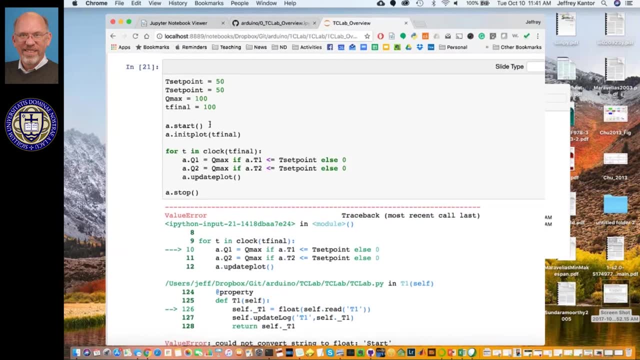 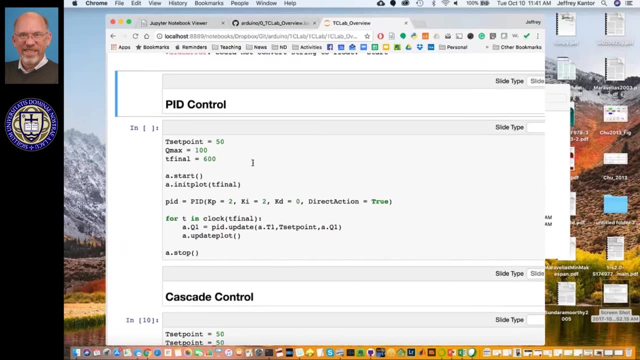 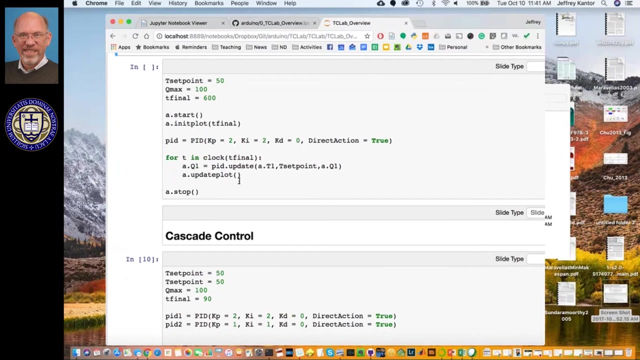 I'll interrupt that current operation and I'll start it again. Oops, Well, we'll move on, And then I'm just going to show you additional simulations that we have working at this point. This is an implementation of a PID control. We've got under development a PID module that will also fit into the PC lab module that I've been developing. 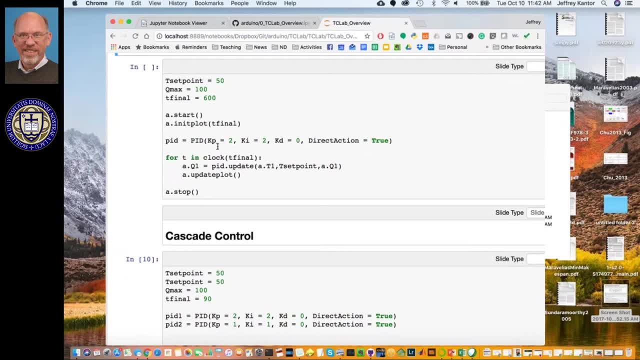 This allows students access to a PID controller, And in the course of this semester, I expect students to be initially coding their own PID controls so that they have a complete understanding of the algorithm, and then later give them access to a professional quality implementation of a PID controller that they can then use to configure different kinds of control strategies. 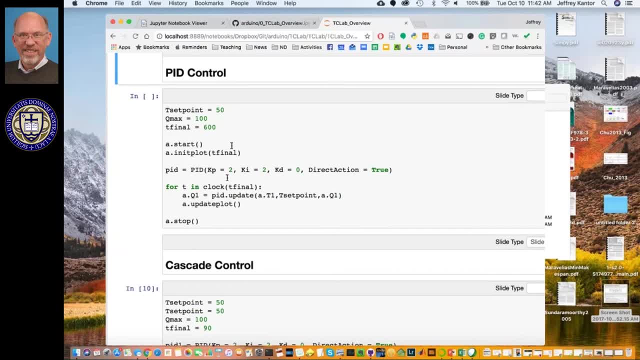 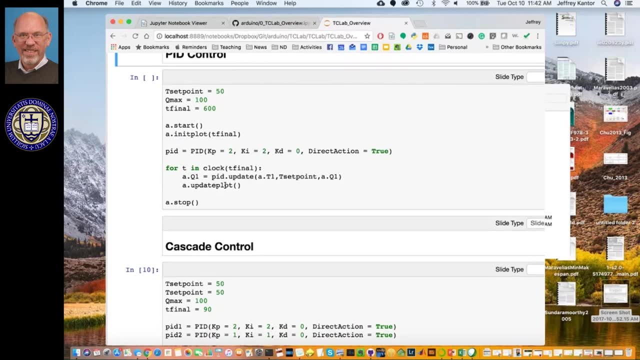 So in this first panel I'm showing how a student could use the PID control module within these labs. So here Q1 is under PID control, using temperature measurement T1 and the set point to T set point And, for the purposes of anti-reset windup, have access to the current Q1 reading, should it be different than the applied Q1.. 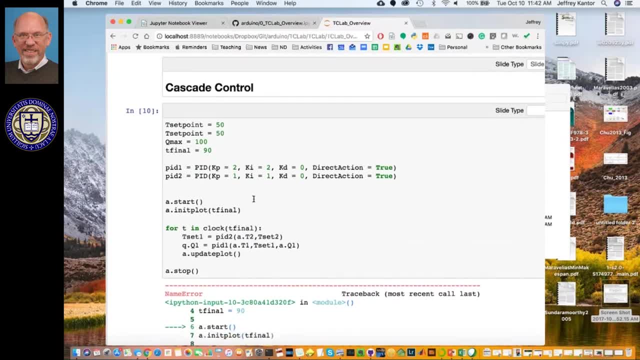 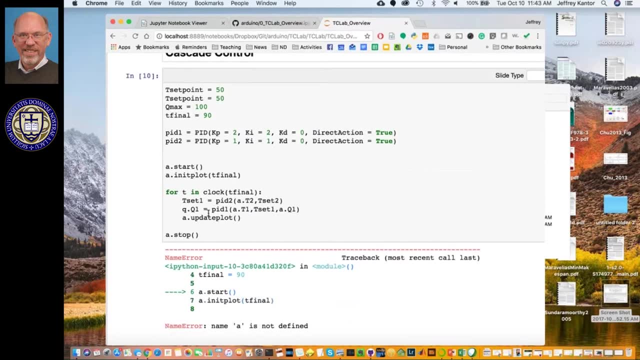 And then in the second panel I have a demonstration of cascade control, where one controller is used to provide tight control around Around the first temperature sensor using heater one, And the second controller adjusts the set point to the lower level controller in order to maintain control of temperature T2.. 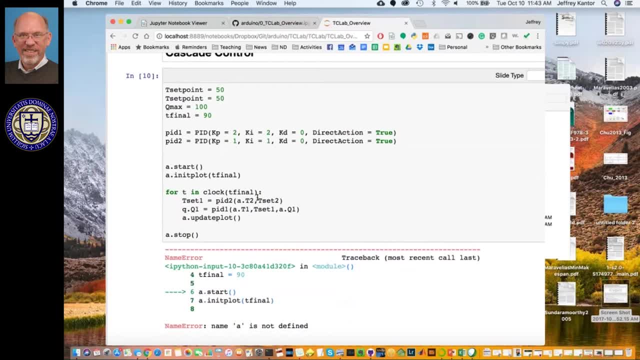 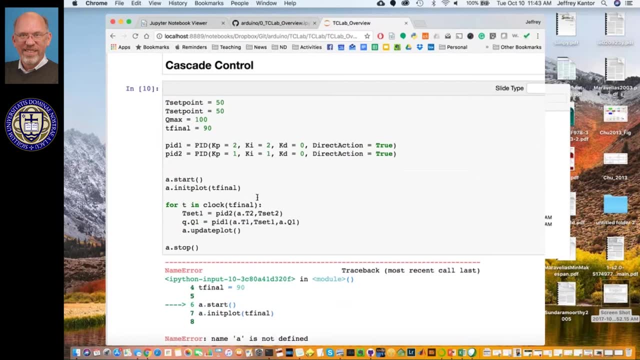 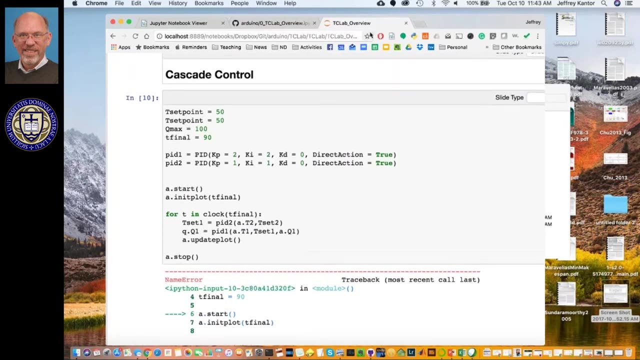 I find that teaching concepts like cascade control can be challenging, and so I'm pretty excited about having this ability to demonstrate cascade control in a lab setting. So here's Q1.. So with that, John, I'll turn it back to you. 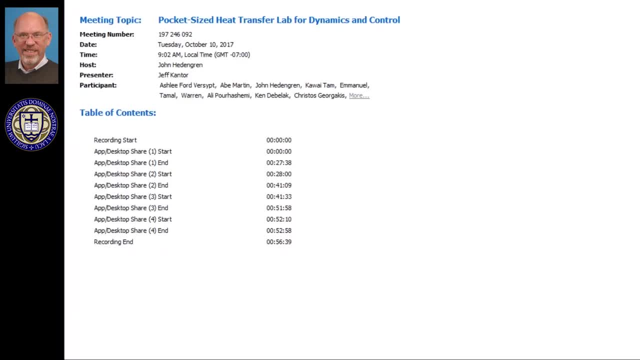 I'll turn off my screen sharing. Okay, great Thanks, Jeff. And one of the things I think that's a key thing from that is that these labs are really customizable for those who would like to. you know, basically take the lab and then make it their own and adapt it to the needs of their course. 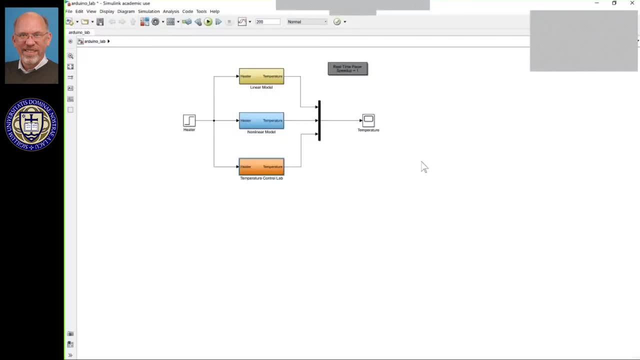 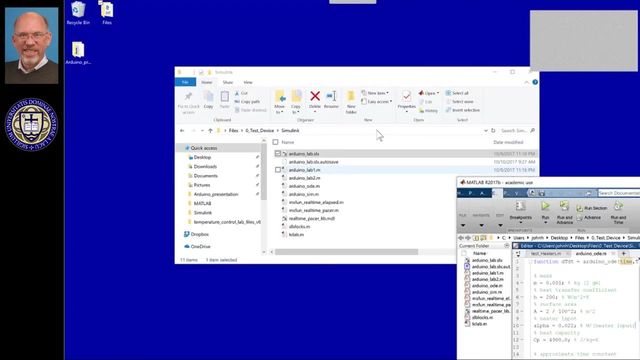 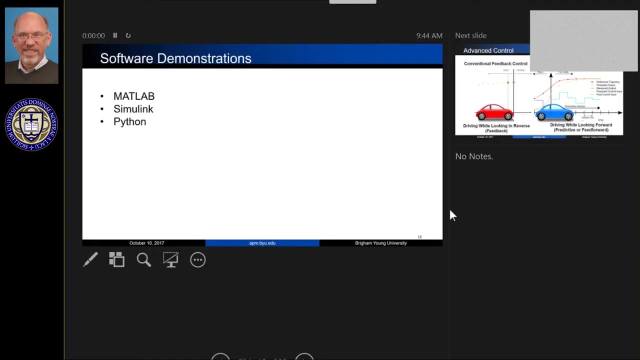 So we've certainly done a great job of demonstrating how it can be customized. Let me go ahead and just open and close my Simulink and go back to – there's just a couple additional slides that we had, some additional modules that we have developed. 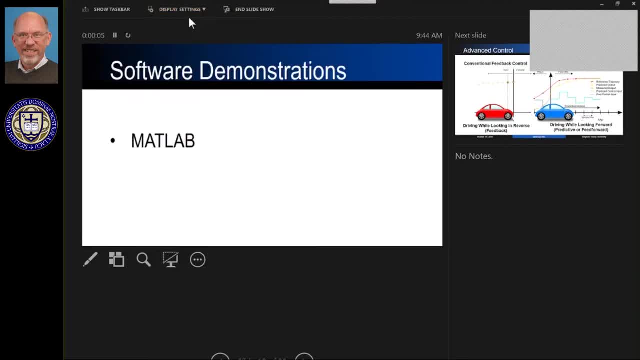 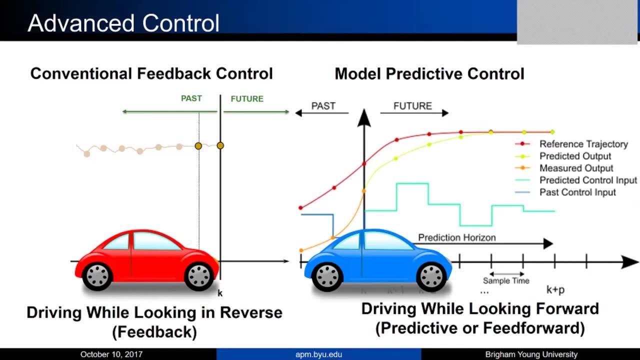 And let me go ahead and just switch this again. Okay, So we have model predictive control as well, Some estimation Like Kalman filter, Kalman filter moving horizon estimation, Identification algorithms as well. This is a MIMO system: multiple input, multiple output. 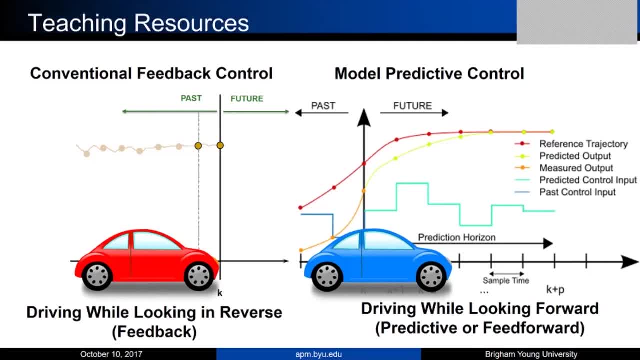 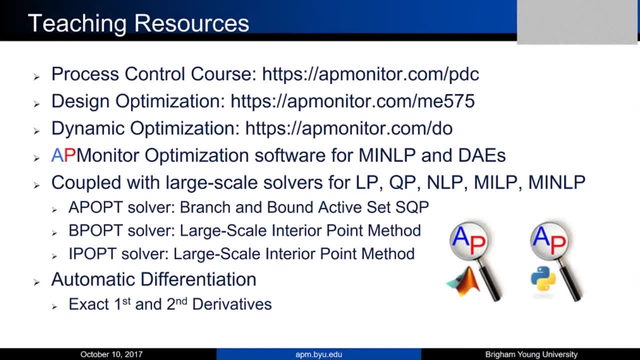 So you can do single output- single output or multiple input- multiple output. There's also some teaching resources. I have a process control course that I do in Python and Jeff has his content that he showed you there as well- and also for optimization and dynamic optimization. 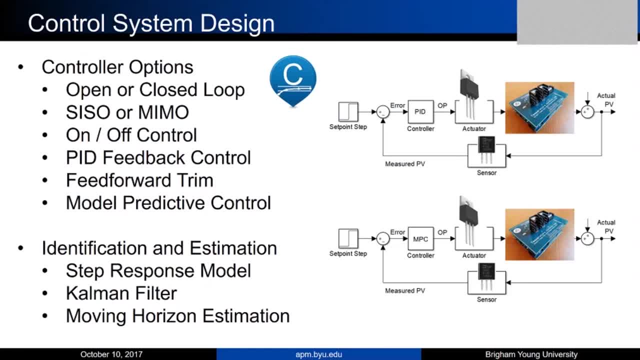 And basically we want to just give some resources, some starting code. Some may not have the time to put into developing some of these, and so we want to make this a community effort as well. So as we develop things, we'll put them onto the GitHub site. 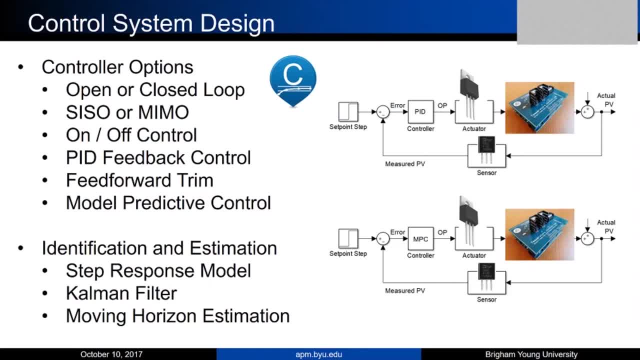 and then you can take that as a starting point or further modify it and then recommit some of those changes back to the GitHub if you'd like. But there are some of the modules that we have already developed and continue to develop more Okay. so just a final thing before we ask if there's any questions. 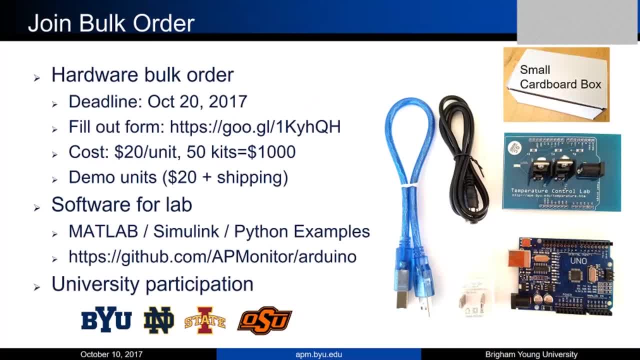 but also just mention that we're putting in a bulk order and one of the main outcomes of today is just get a level of interest on who would like to join the bulk order And you can see the form address right here. If you go there, it's just a Google Doc. 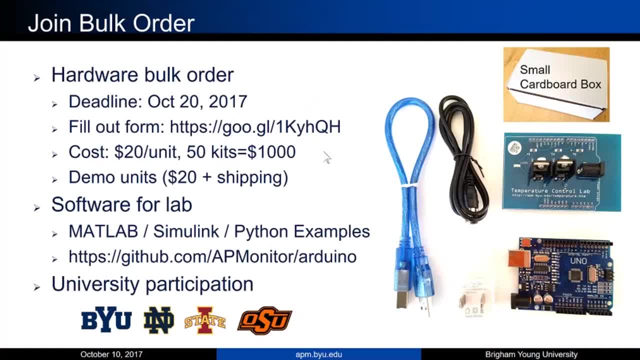 It's like a questionnaire and you can fill that out and provide some feedback about what your level of interest is and how many units you might want. I know some of you are still trying to work with department chairs and others to try to get some funding for this. 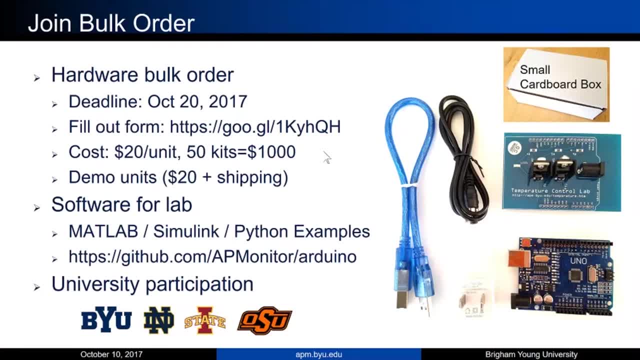 and so we're trying to have a target date of October 20th to be able to ship that off and hopefully get those units back by early December and get those into your hands. We have another bulk order that we just put in. It was 500, and more than half of those were already spoken for. 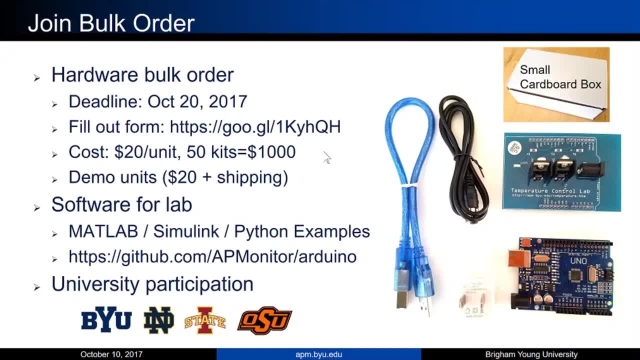 So for those who put in their name that they want some, we'll try to fill those as quickly as we can. Those will be early, well late October, early November that they'll hopefully arrive And we also have a bulk order. 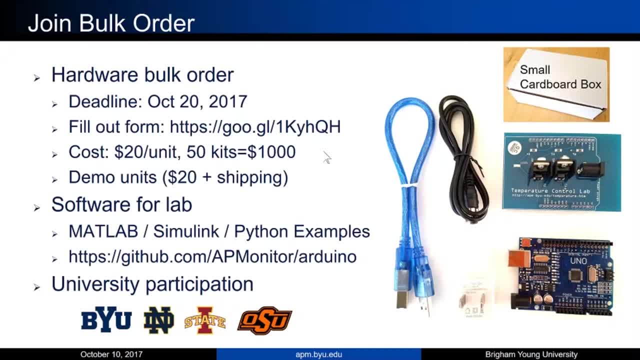 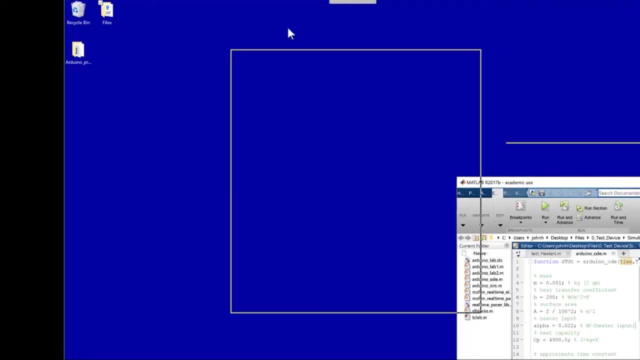 We also have the – okay, so we have a few universities that are already doing that. So let me just show you that form. You can just take a moment to open that up and fill that out, or you can do it after the webinar as well. 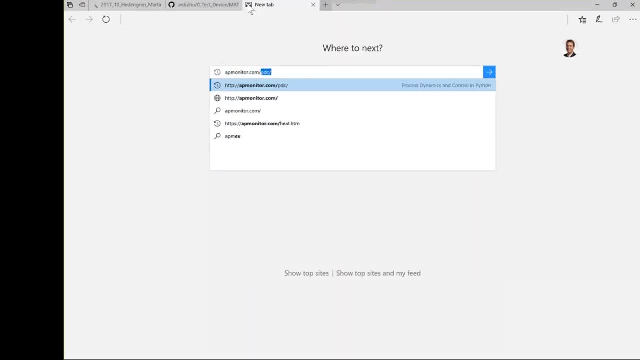 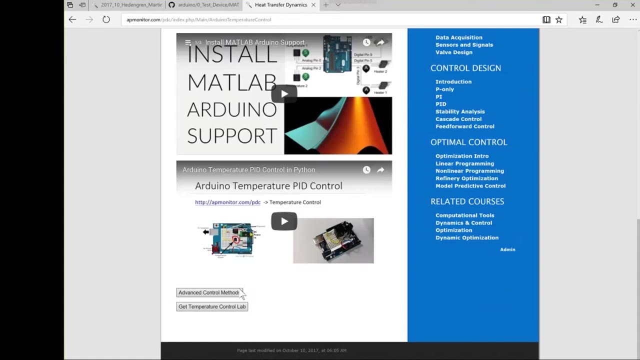 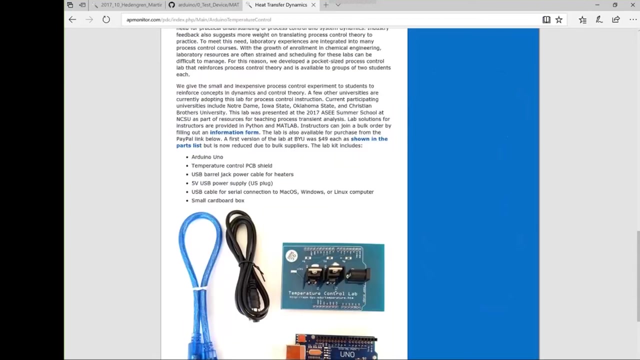 It's just at the apmonitorcom slash heat dot htm. That's the address, And then down at the bottom there's the get temperature control lab And then there's the information form that you can fill out. There's a link right here. 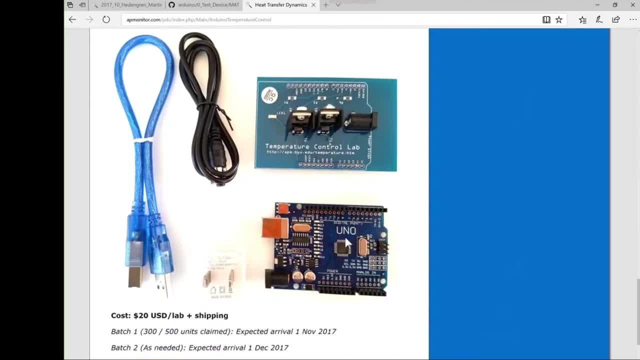 And this one comes with – there's an Arduino Uno that it comes with. It comes with the temperature control lab shield. This is a barrel jack USB. It also has an independent power supply. So one question we had was to use these labs in class. 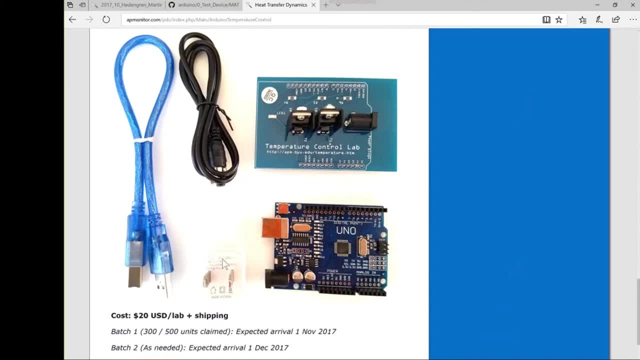 are you going to need power supplies for 50 students in class? The answer is no. you don't necessarily have to do that If you have two USB ports. this one is used for communication right here and plugs into this USB socket right here. 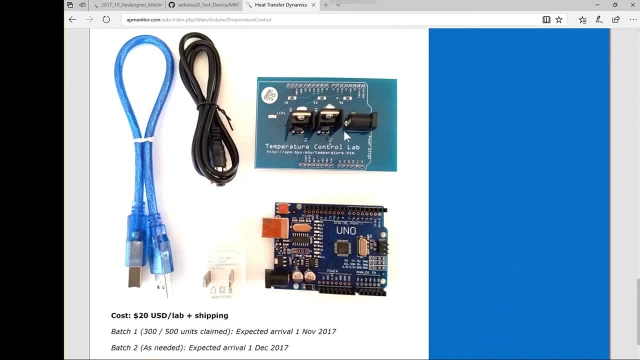 This one right here is the power one and it powers the heaters, And this can either be plugged into the wall outlet or this one can also be powered by another USB connection on a computer. So you just have two USBs going into the computer. 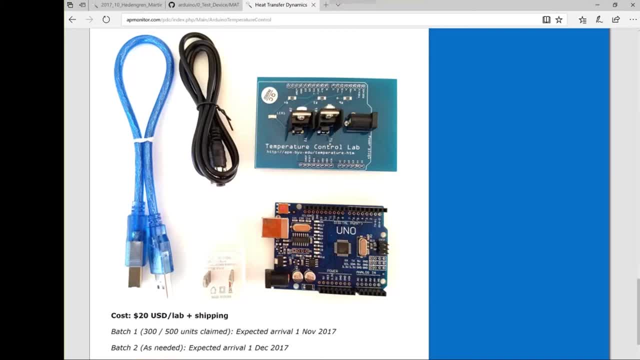 if you wanted to power it and also communicate. We did test some ways to get rid of one of these cords- just have one cable that goes into the computer. But we found that the signal quality dropped because when you start powering the heaters it changes the calibration. 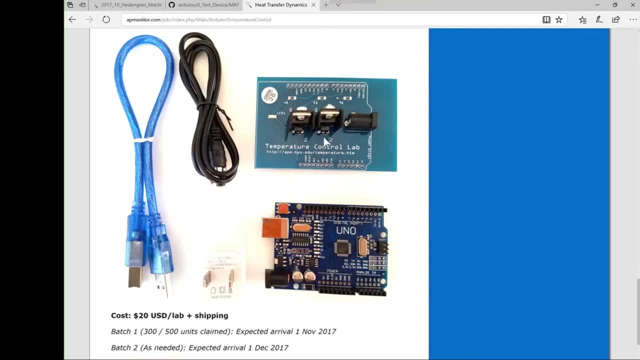 The voltage drops and so it changes how you read the temperature, So we felt like this design would be most flexible. But these are the things, And if you need to do some more work, these are the things that come with that lab. 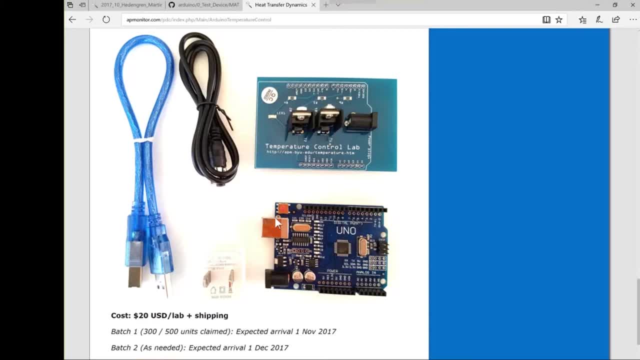 Also a small cardboard box, just so you can kind of manage those. have students check them out if you want. Probably the minimum amount that you'd need for a large class might be ten. Just leave them in a central lab. Students come check them out and use them. 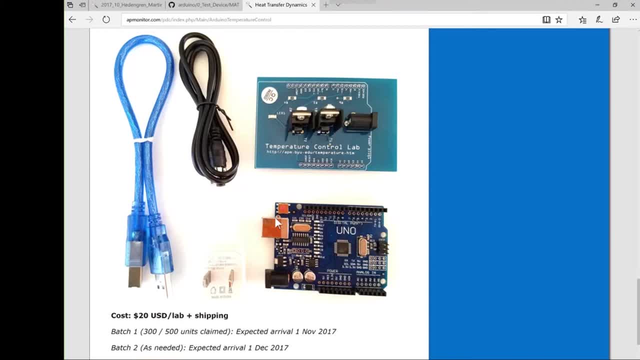 If you want to have more of an individual experience for the students. I find that groups of two work well well. with this one I'm going to have about 50 labs for the hundred students in the class. so with that we'll go have some question answers and you can just. 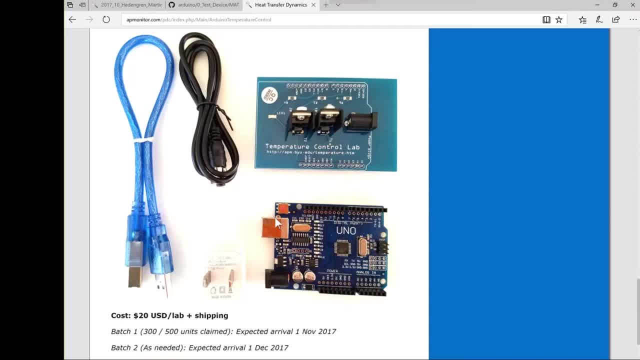 when you ask a question. just if there's one of us that you wanted to ask a question in particular, to feel free to mention that they couldn't unmute your microphone- if you'd like to ask a question or make a comment and we'll try our best to respond to those, okay. so I got a chat. I got a couple questions here. 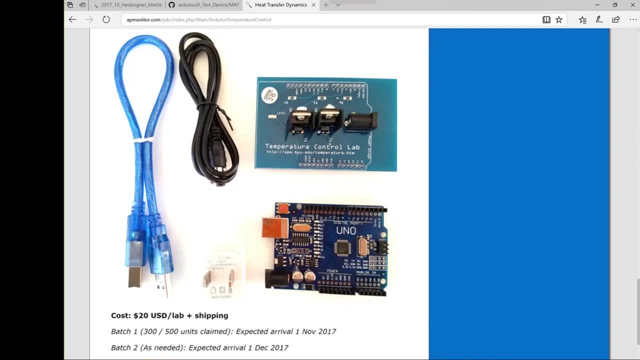 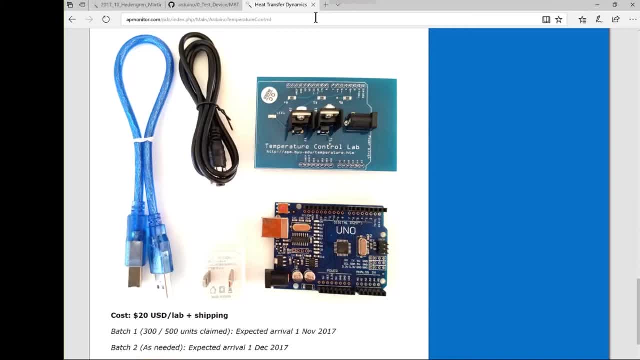 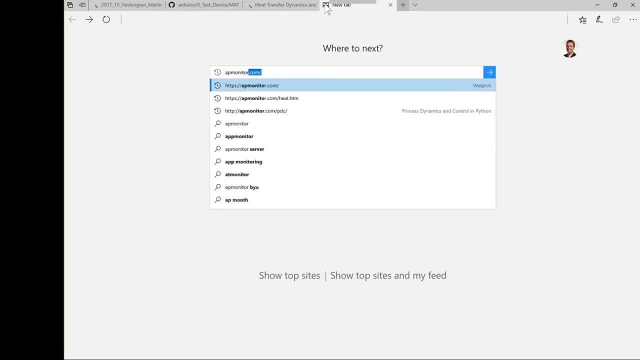 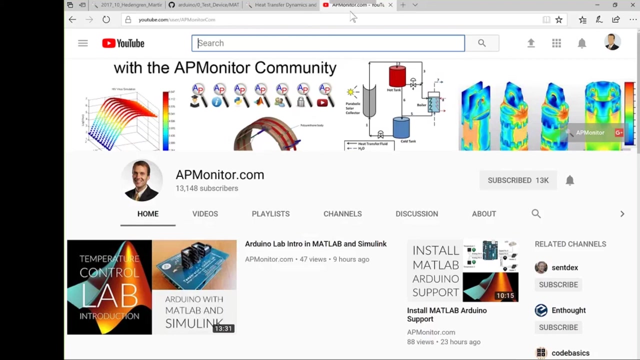 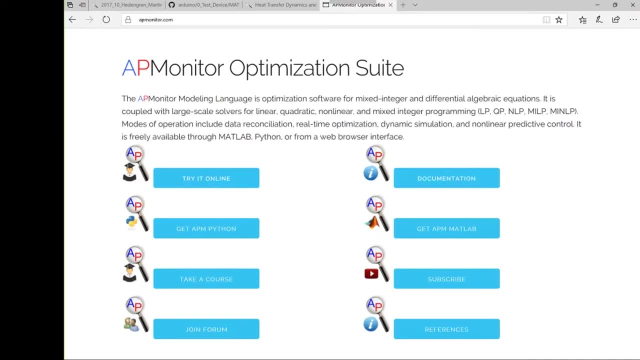 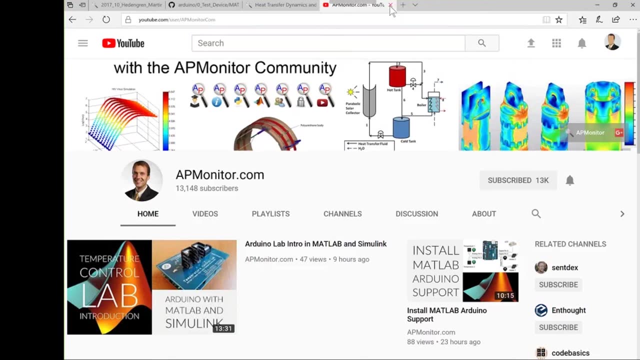 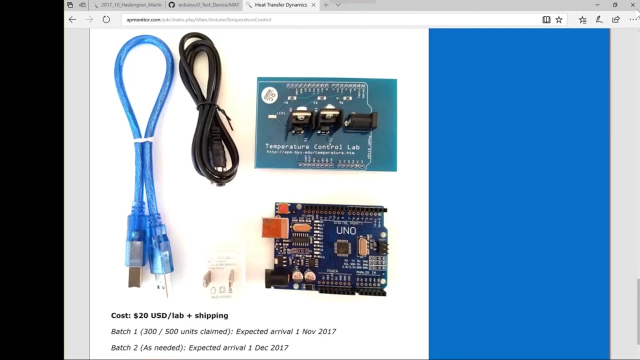 AP monitor comm. there's the youtube link right there and that'll bring you to the channel as well. okay, so I'll post it here on the on my youtube channel, okay. next question: let's see, let me go down. do your computers have serial ports or USB to RS 232? yeah, we just use the USB. 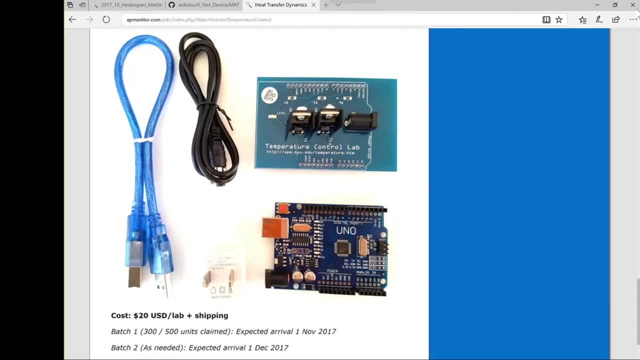 connection for that and we've been able to test it with the Mac and the Windows and, as you saw, Jeff, he has a Mac OS and I typically use Windows. I don't think we've tested it on Linux yet, but no, actually we have. we have tested on Linux. 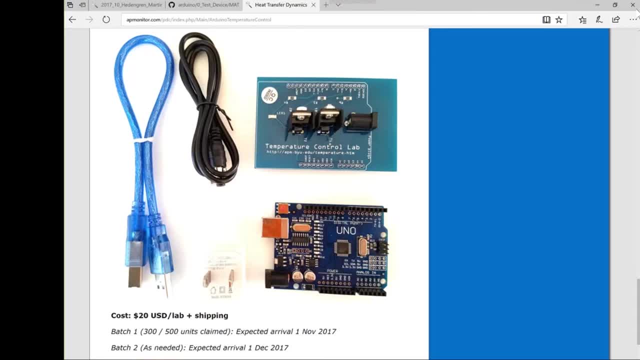 so should work on Linux as well. okay, and the Arduino is connected to the laptop- okay, nearly all our students access Mac and Windows, so we're going to test it on the Mac and the Windows as well. okay, nearly all our students access Mac and Windows, so we're going to test it on. 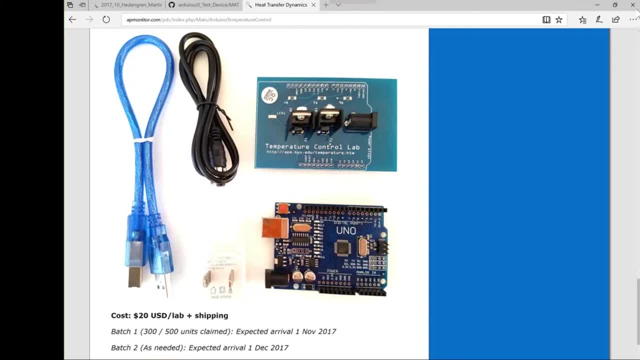 MATLAB Simulink using remote desktop. do you have any experience with that? hmm, I don't. I don't have any experience with the remote desktop, Jeff. what about you? I've seen it used that way. I'm not sure that would be an environment where this would work very well, because Simulink would have to have access to the 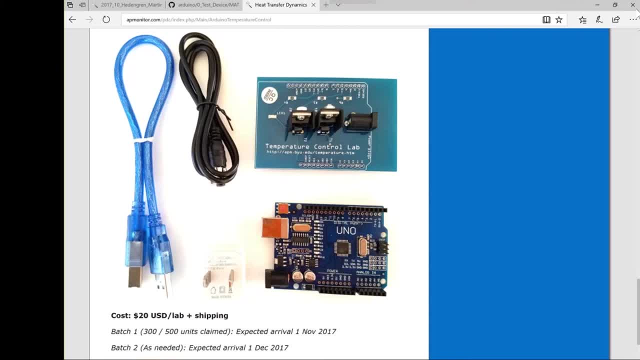 comport, but I don't think it would. through a remote desktop, I don't, unless you're thinking about having the device remotely as well. yeah, that, yeah. if it were remote to the desktop or to the computer, that was access you were accessing through the remote desktop, then it might. yeah, I'd be a little leery. 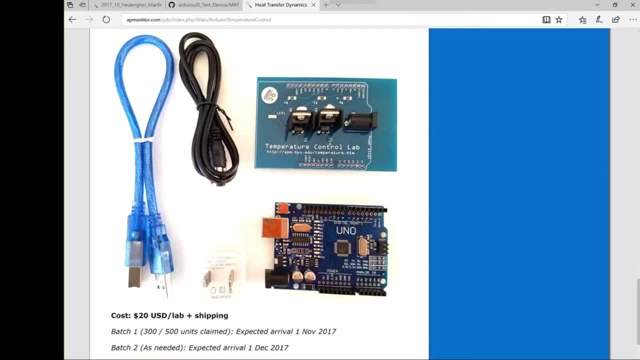 of that, because the devices do get hot and I'd hate to have something a remote location of getting hot and outside of you know. you know outside where you're, you know direct manual intervention, mm-hmm, yeah, I agree with that. okay, so another question: can we change PID parameters in Simulink and how long does? 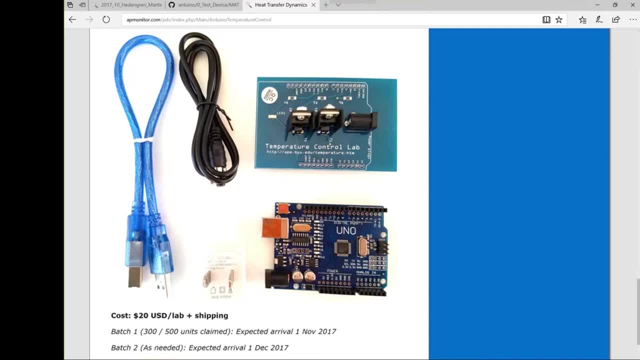 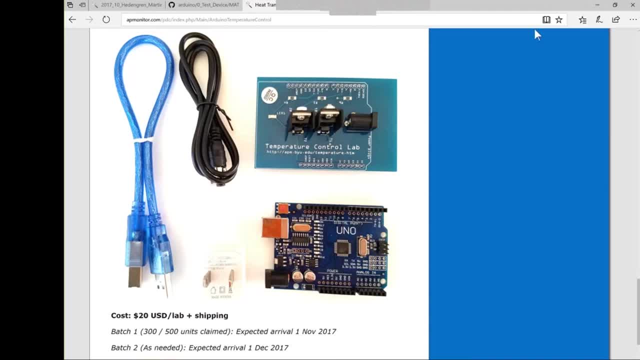 from here. so I am going to start my. let's see, I'm going to start my video again and and put myself on speak. okay, so here is the lab that I've showed you guys before. there's also one of the earlier versions of the lab is right. 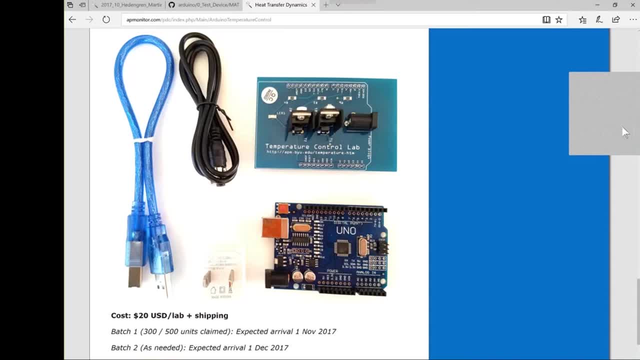 adhesive between the heater and the temperature sensor. So one way to decrease the time constant is actually to bind those two And it'll decrease it to maybe about 100 seconds or so for a time constant. With the lab right now it's probably about 150, maybe 200. 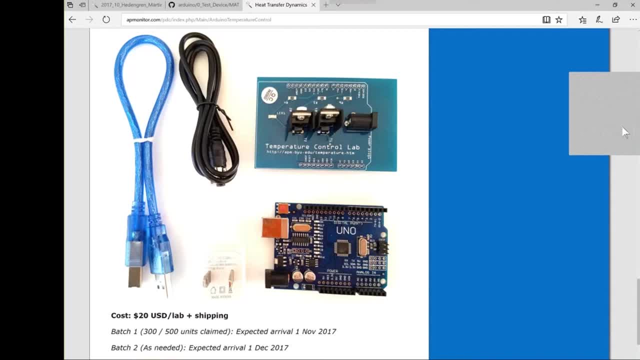 seconds for a dominant time constant. So a step response might take four minutes or so, But you kind of saw that with Jeff when he was stepping it up. It might be two or three minutes to do a step. John, I have an experiment running in the background. 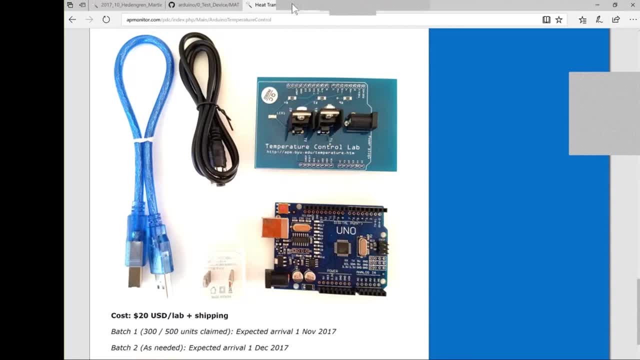 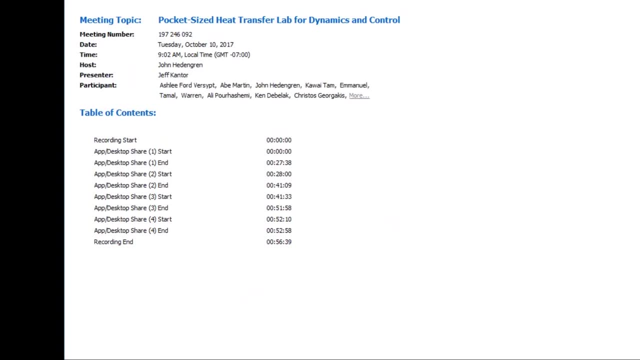 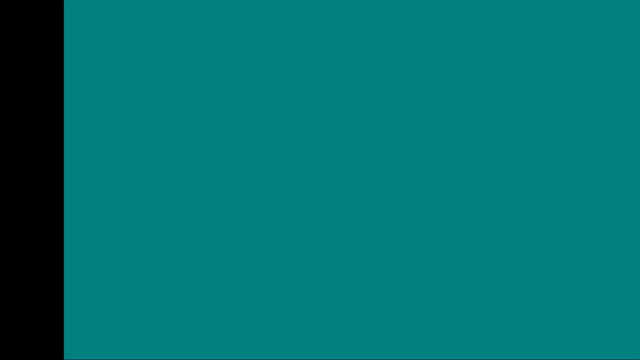 If you could switch to my screen, I could show you the time constant. Yeah, OK, OK, You should have privileges now. OK, All right. so what I have is: can you see me? OK? So what I've got going on here right now. 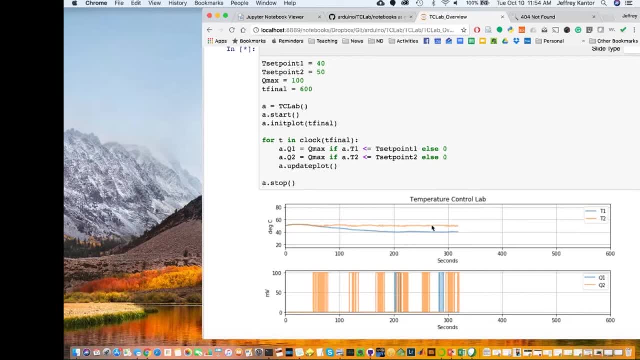 is control of both the temperature, T1 and T2.. I'm using on-off control on each of the two loops. You can see I started it up about five minutes ago while we were talking And you can see it takes about 200 seconds or so. 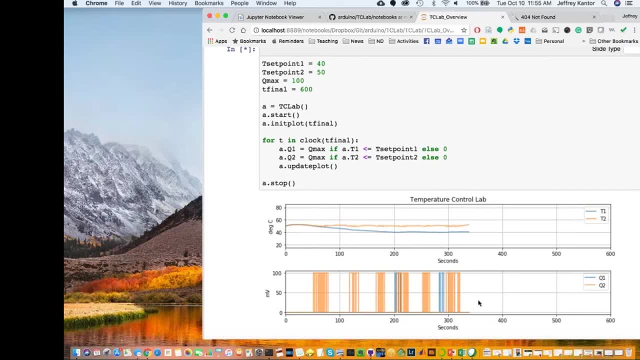 to get to steady state And you can see below. You can see the switching that's going on. Because of strict relay control it's a little sensitive to noise, So this would be an example where you could tell the hysteresis would. 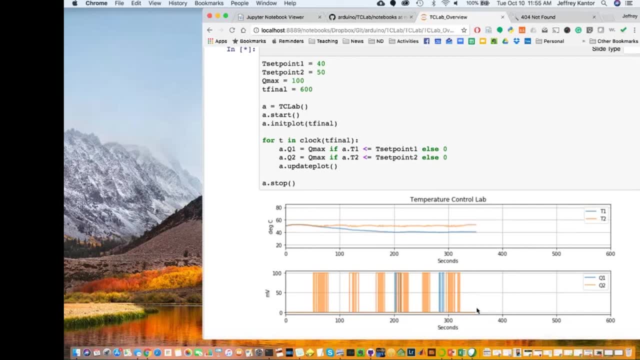 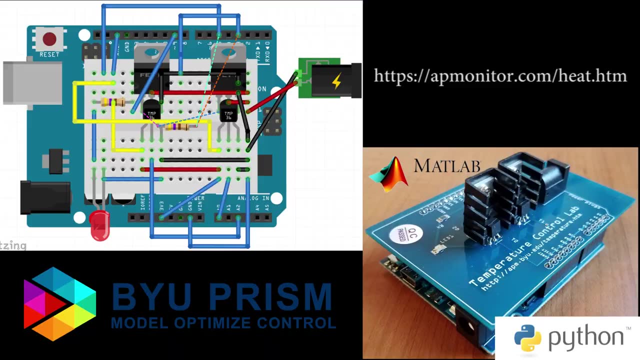 be helpful in the control loops. So there's a lesson to be learned there too. But this gives you a sense at least of the time constant. OK, great, OK, I'll give it back to you, John. OK, and so just another question. 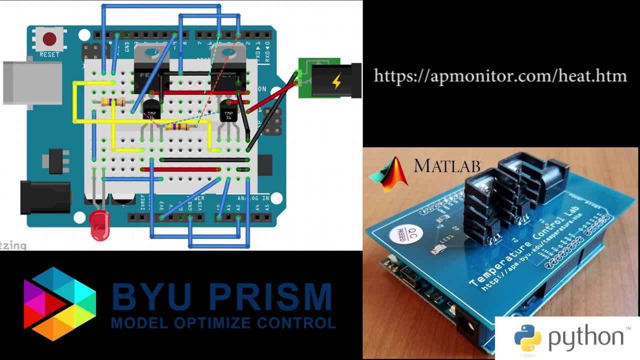 that came in through the chat. So we are using the instead of the. you know the, of course the official version of the Arduino. we're using a generic version. They seem to work fine. We've had multiple hundred of those. 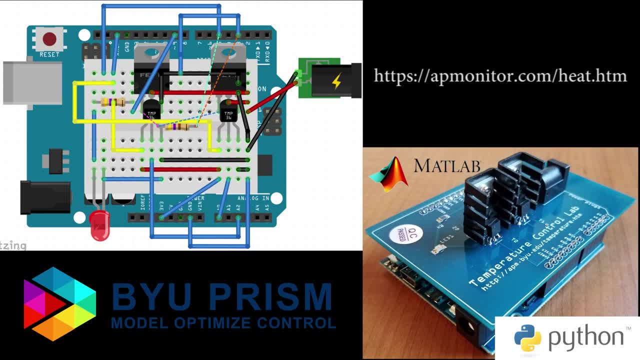 used by other labs in our department, And so it makes it less expensive. Part of the reason why this lab went from $50 down to $20 is that we were able to use less expensive versions because we don't have students doing the wiring themselves. 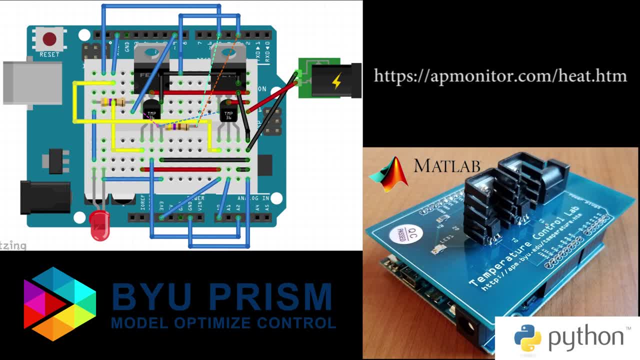 So we needed the more expensive version, like a rugged Arduino Which has circuit breakers and other things built into them, Because it's a fairly it's the chance of damaging the Arduino device itself is much lower. So we do have Arduino UNOs or H-Duinos. 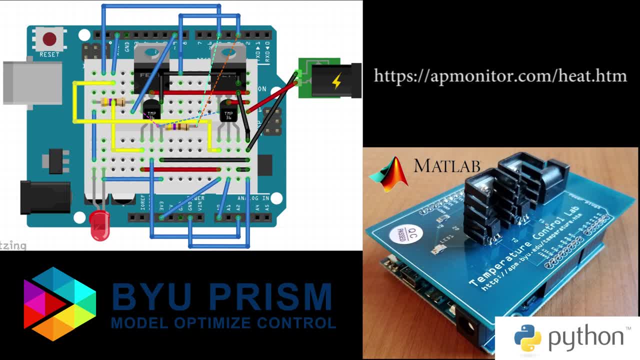 Both of those should work OK. another question we had: What if I want three modules this time and probably purchase more later after trying it? What is the price for three modules? So they're just all $20 each. You can order as few or as many as you want. 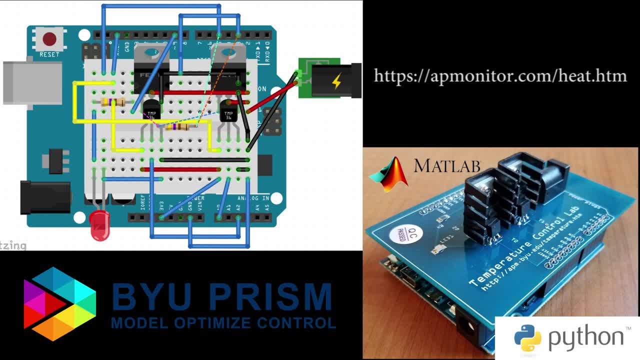 The main thing is just getting in on the bulk order, I'm probably only going to do one bulk order after the first 500 that come in. So it's just if you do want 50 at a later time and it's not part of a bulk order. 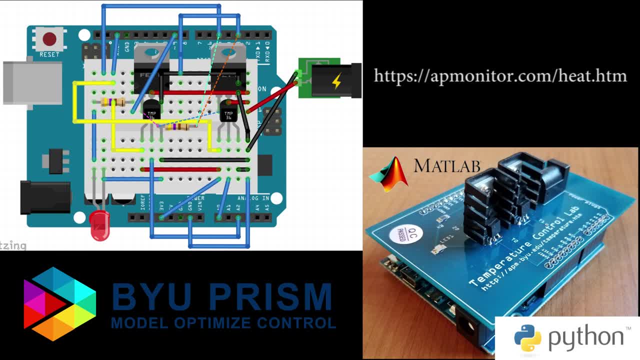 then it might be next year before you get some. So three is fine. Just on the list. you can either. You can either order one through the Buy It Now through the- there is a button down there- through PayPal, or I can send you an invoice. 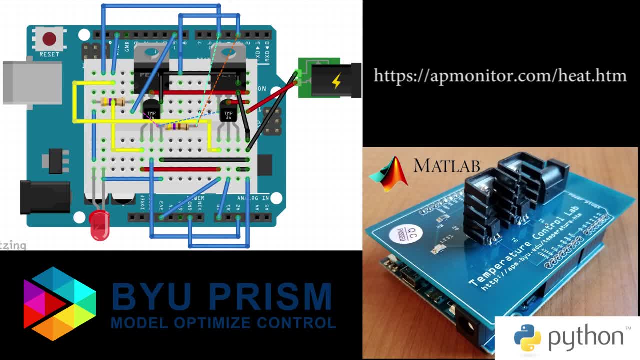 OK, looks like Rick was able to offer some advice on. you can share local ports with a remote desktop session. You may need admin privileges to make it work, And then he included a link that shows how that would work. So it looks like you can with remote.